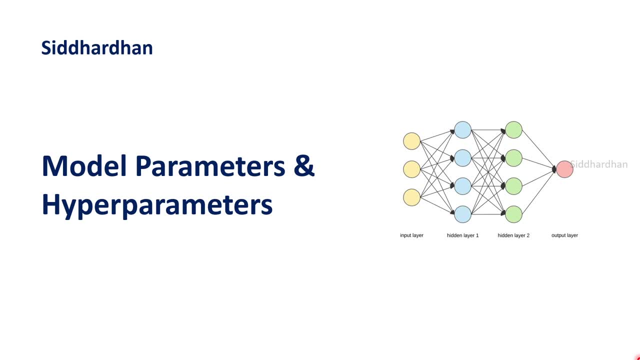 the intuition behind the different types of model that we have and how we can build these models from scratch. So it's a good idea to discuss about the parameters before going to that part. So that is the idea behind this particular video. So let's get started. 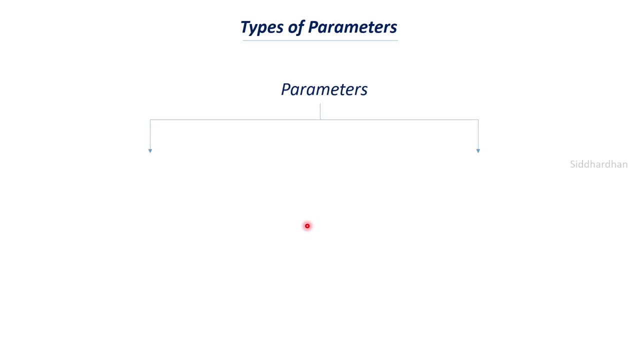 So, as I have told you, the two main types of parameters that we have in machine learning are model parameters and hyper parameters. So I will give you the definition of these model parameters and hyperparameters. Model parameters are the parameters of the model that can be determined by training with. 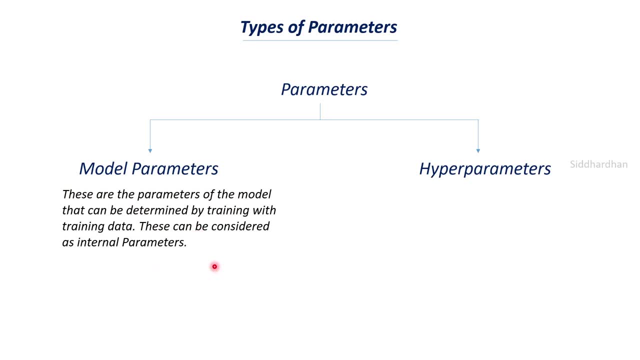 training data, So these can be considered as internal parameters, and the two important model parameters that we have are weights and biases. okay, So this is the definition of model parameters, and the two model parameters are weights and bias. Now let us try to understand this definition. 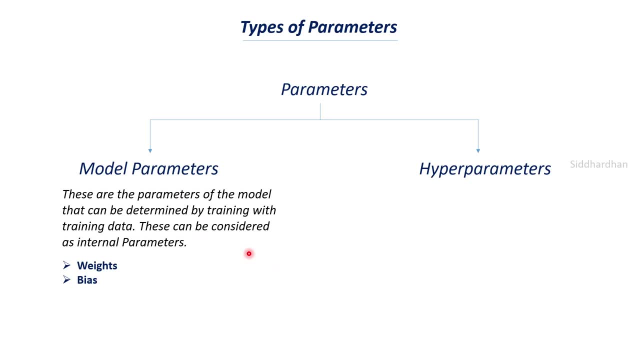 So in my previous videos I have made several videos on the topic linear regression. right, and we know that the equation of a line is: y is equal to mx plus c. So I have written the same equation here. I have just replaced m with w and b with sorry, the c with b. okay, 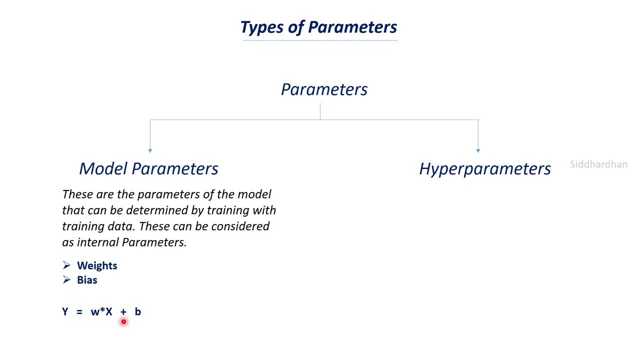 So y is equal to mx plus c is written as: y is equal to wx plus b, where m represents the slope and c represents the intercept. So I have replaced m with w and c with b, So it is actually the same thing. 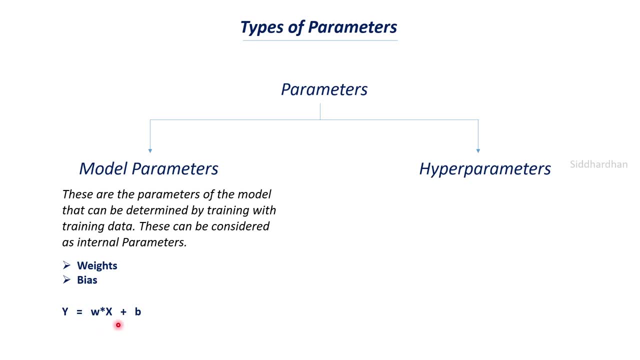 Now we know that whenever we are training a model, we will try to fit this particular model to the data that we have right. Say, for example, Let us say that we want to build a model, build a linear regression model that can predict. 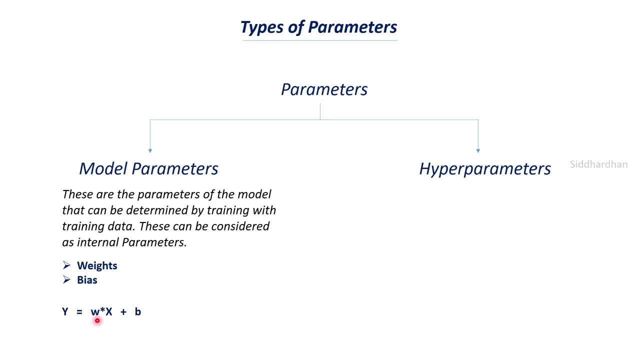 the salary of a person based on their number of work experience. So in this case, y will be the salary of the person and the x will be the number of years of experience for that particular person. okay, So what we will try to do is we will try to fit this data. 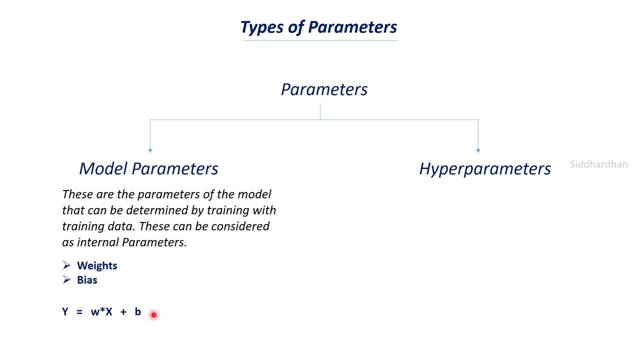 Let us say that we have about 100 data points. So we have a data of 100 different people regarding their number of years of experience and the salary that they are making. So we will try to fit this particular data to a linear regression model. 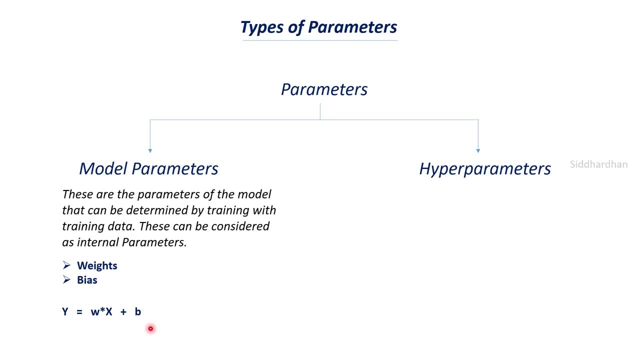 And the normal regression is nothing but a simple straight line. okay, So in that case we will get a straight line with some parameters. So it will be: y is equal to mx plus c, And for that particular data we will get some slope values. 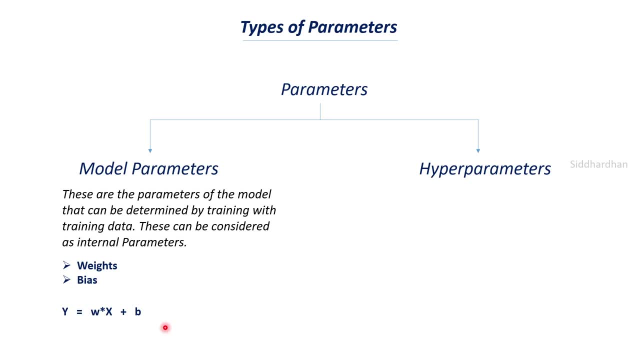 Let us say that slope value is, you know, 30 or something, and we will get some intercept value. Let us say that intercept value is 3 or 4, something. Okay, So these can be any values. This slope and intercept value, m and c value varies depending upon the data. 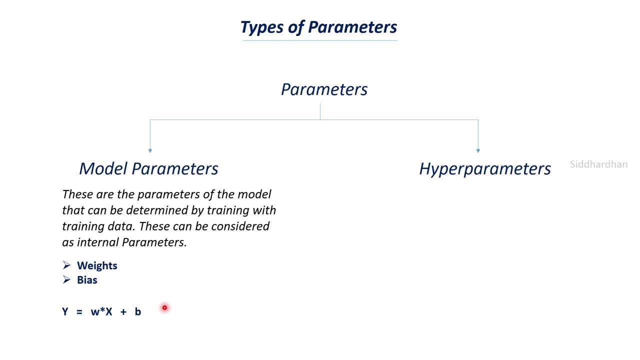 So it won't be a constant in all the cases. So this particular values differ in all the cases based on the data that we have. so in this equation, as i have told you, the m is replaced by w, so the slope is replaced by weights and intercept is replaced by bias. actually, these are the same. 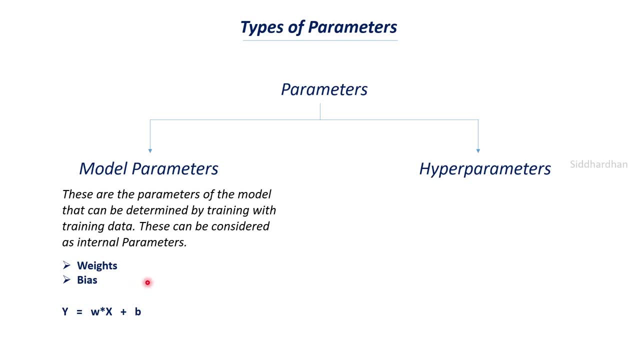 things. so slope and weight represents the same thing and the intercept and bias represent the same thing. so i'll tell you how this is, and now you can see this definition again. so these are the parameters of the model that can be determined by training, with the training data as i have. 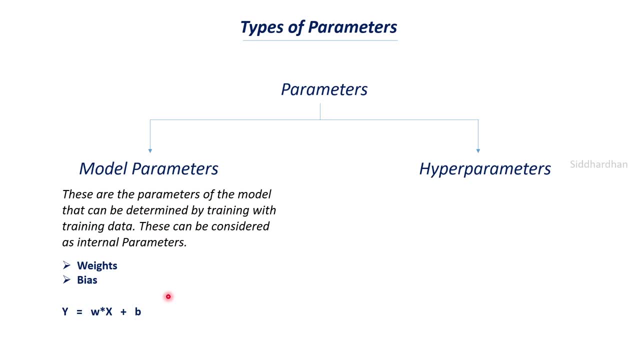 explained you in this example. so we will get this slope value and intercept value after fitting the data to our model right. so the model parameters are those which are obtained after training the data. so hence these are considered as internal parameters because these are the parameters within the model, right. so these are the parameters of the model. so for a line, the 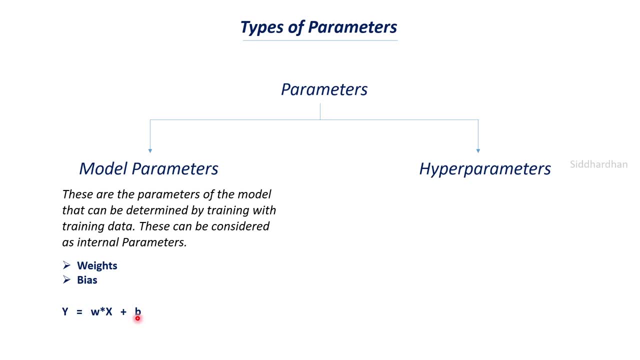 parameters. the two parameters are slope and intercept, or you can call this as weight and bias. so these two will be the model parameters and we can call this as internal parameters. now let's try to understand about the hyper parameters. hyper parameters are the parameters whose values control the learning process. 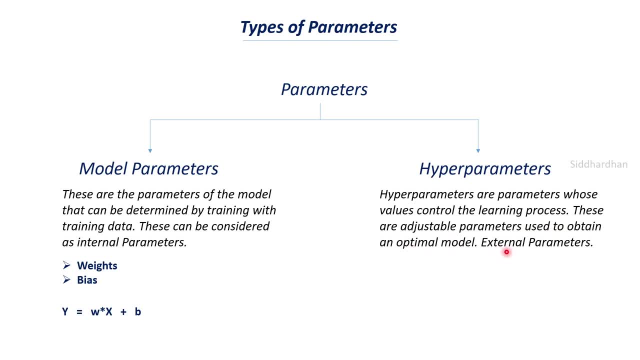 these parameters are the parameters whose values control the learning process, are adjustable parameters used to obtain an optimal model, and hence these are called as an external parameters. now let us try to understand this particular definition. So, whenever we are fitting a set of data to a linear regression model, what we will do is 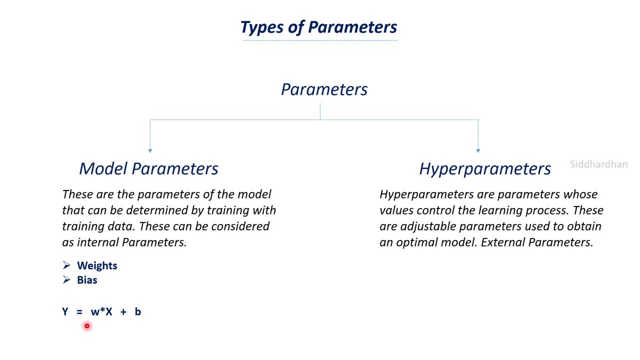 we will try to iterate the process. we will try to fit the data multiple times in order to get the best values for the parameters. so in this case we have the weight value and bias value right. so we want to get the best values for this weight and bias. so there may be some errors, so error in the 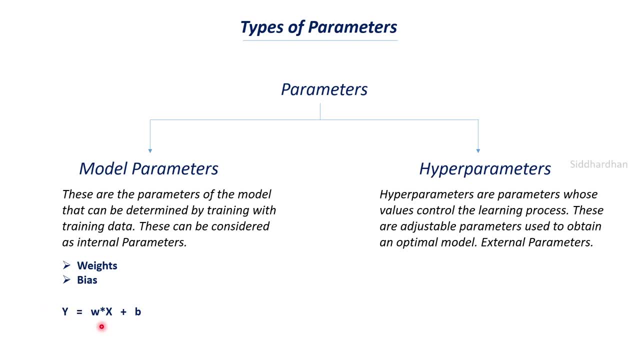 sense, let us say that we get a linear regression model with some value for weight and some value for bias, so this model cannot make better predictions. so in that case what we will do is we will try to optimize the model to get a better accuracy score, to make better predictions. 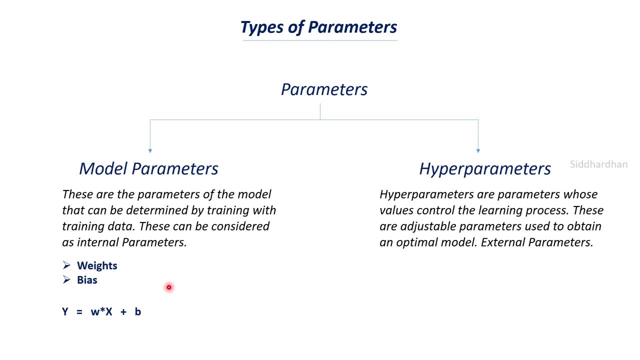 so in that case, what we will try to do is we will try to reiterate the model with that particular data. so we will try to fit the data again and again to the model until we get the best value for weights and biases which can give you accurate prediction. so in that case, what we will do is we 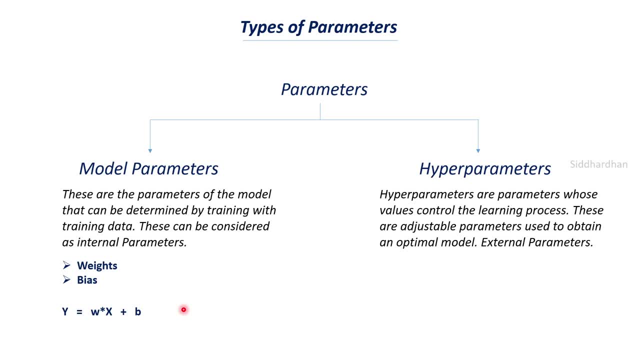 will try to manipulate the values for the hyper parameters. so example of this hyper parameters are learning rate and the number of epochs. so every time you reiterate the data, what happens is we will try to change the values of weights and bias slightly. okay, so we will try to give a slight variation. 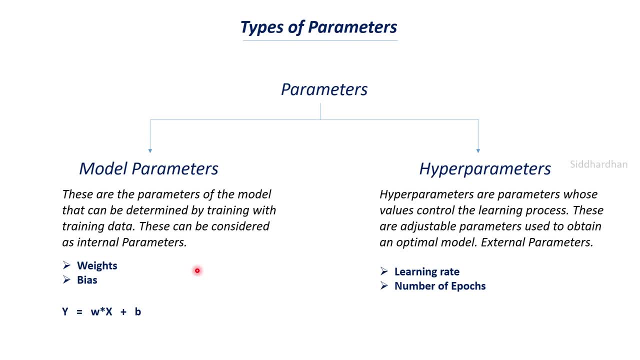 to the weight and bias and we will try to check the prediction of the model. okay, if the model make a good prediction, then we can say that it is accurate model. if the predictions are not proper, then it is not very accurate, right? so there will be a particular change in the values of weights. 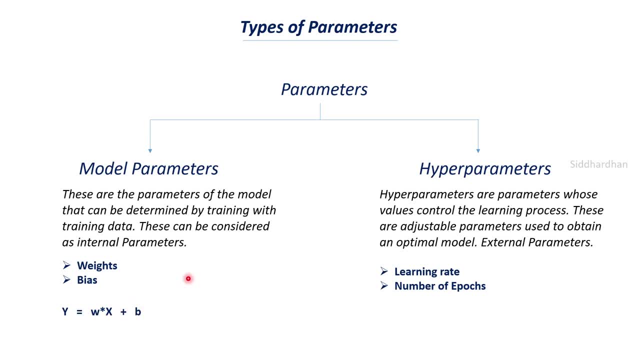 and biases in each iteration or each process that we do, and this change that we are giving is called as the learning rate, okay, and number of epochs. number of epochs represents the number of time we are training the model with that particular data. let us say that we have about 10 iterations. 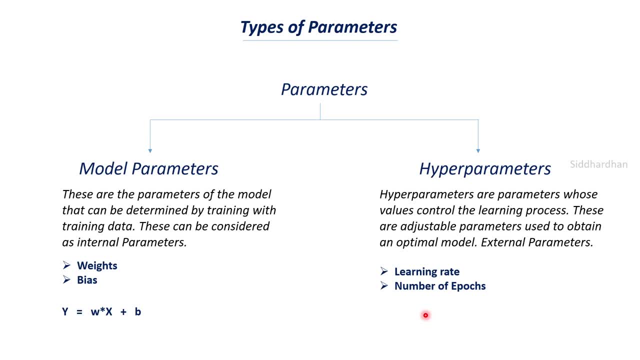 so we want the model to go through the data 10 times, so in that case the number of epochs will be 10. okay, so this is about the learning rate and number of epochs, where learning rate represents the amount of change that we are imparting to the parameter values. 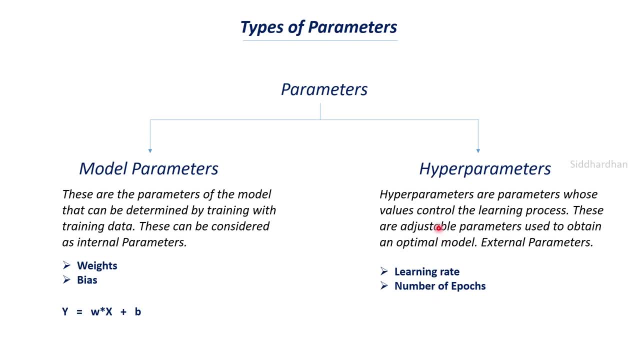 and number of epochs represents the number of iterations that we want. so now you can see the definition again. so hyper parameters are the parameters whose values control the learning process. so learning process is fitting the data to the model. and these are adjustable parameters because we can adjust the learning rate and the number of epochs, so we can manually give the value. 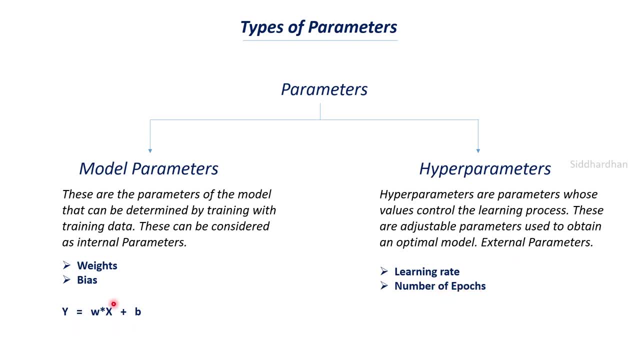 for learning rate and number of epochs, whereas we cannot give the values for this- weights and biases- the model has to determine the value of weights and biases depending on the data. so that is the difference between model parameter and hyper parameters. as i have told you, it is used for 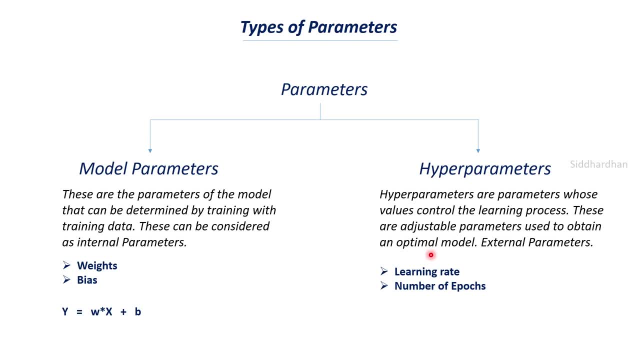 finding an optimal model. so an optimal model is something that make accurate predictions and better predictions. so this is the use of hyper parameters, and these are external parameters because they are not within the model, so these are not the parameters of the model, but we are giving separately, so we are giving manually, these values of learning rate and number of epochs. so these 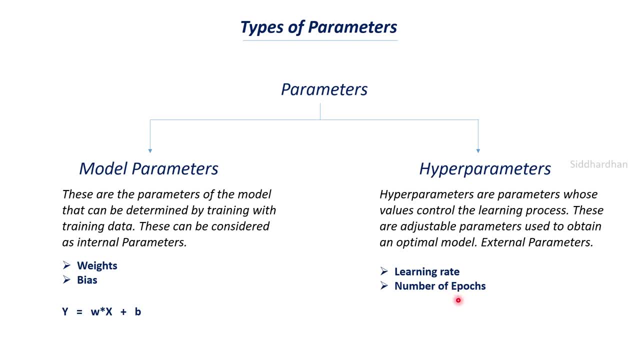 are the two different types of models that we have in model parameters- sorry, in machine learning models. so one is model parameters, which are the model parameters, which are the model parameters, are the parameters of the model. and then we have these hyper parameters which, uh, you know which. 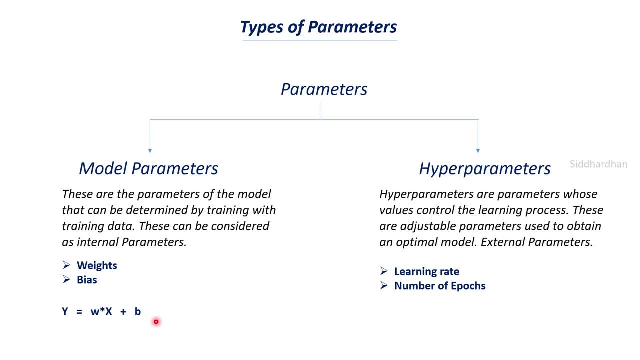 determines the learning process. so how much change you want to give to your weights and bias and how many number of iterations you want to give to your model. okay, so these are the two main important parameters that we have and, uh, you know, apart from this learning data, number of epochs we also have. 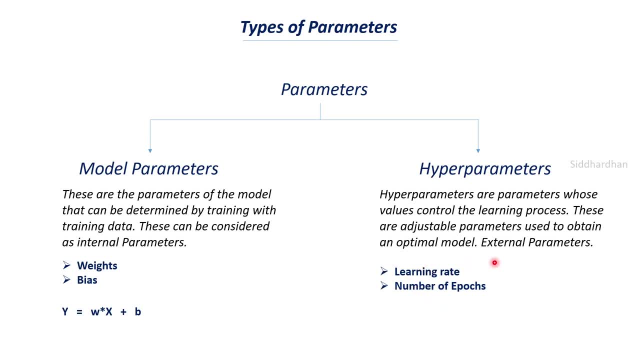 some other hyper parameters, but these two are the main things that we will, you know, regularly use. now let's try to understand about these uh, weights and bias and learning rates and number of epochs separately. so wait, so what is meant by the weight of a model? so i am sure that if you are trying to 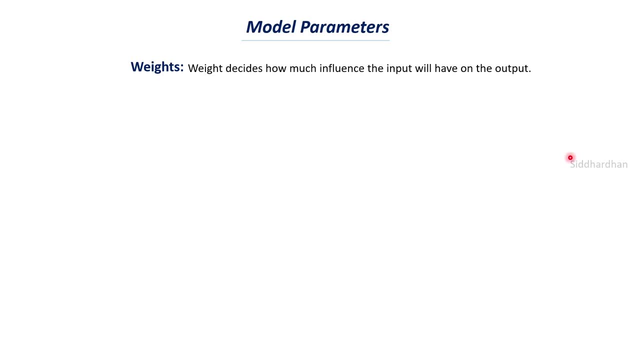 learn machine learning. for some time you would have, uh, come across these words, weight and bias, but you may not have a clear understanding of these two terms. now let's try to understand them. and these are very main, important concepts when it comes to machine learning. so weight: weight is a value, so weight decides how much influence the input will have on the output. 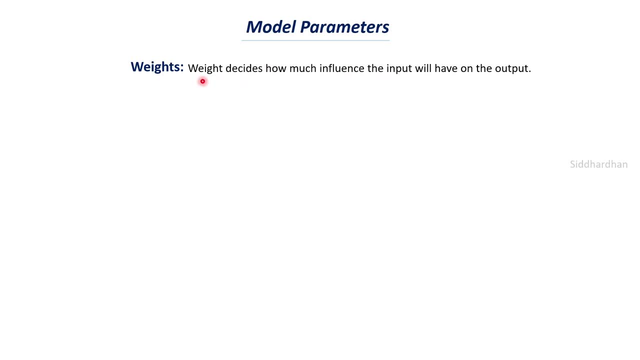 okay. so just read this definition again and you can take a note of that. so this is very important. so in a data set we may have, you know, several features, so and you can have a target variable as well. let's say that let's consider this particular data set. so in this i 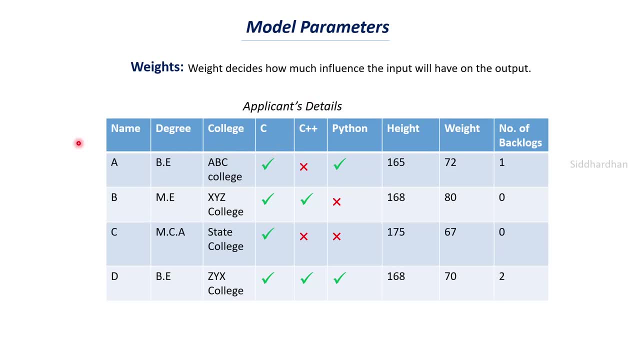 have given data regarding an applicant for a job. let's say that we are building a machine learning system that can predict whether a person can get a job or not, based on some parameters, based on some features. so in this data set, we have the name of the person, the degree that they have, their 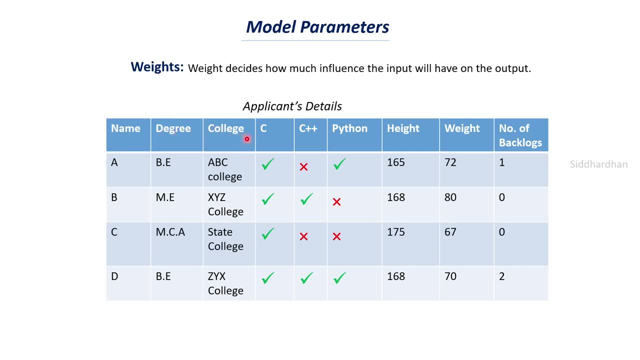 educational qualification and the college from which they have studied it, whether they know c programming and whether they know c plus plus or python. and what is the height of the person, what is the weight of the person and number of backlogs, whether they have any areas or not. so this is the data that we have. so how many features do we have here? so one is. 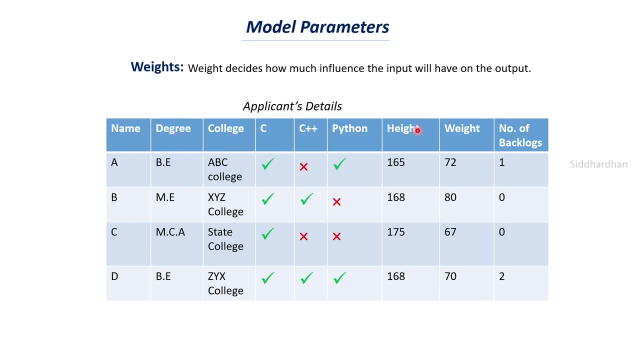 name: degree, college, c, c plus which python, so seven, eight and nine. okay, so totally, we have nine uh features in this particular data set. okay, so each column represents one feature and the target variable will be whether the person will get a job or not. one type of uh. the target will be: yes, the person will get a job, and the other type of the value, 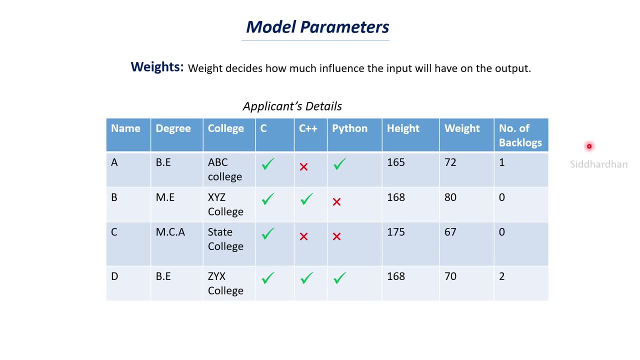 which we can have is no, the person will not get a job. okay, so that will be our target variable, and these nine column represents our features. now we need to find whether a person will get a job or not by analyzing this particular data. now, all these columns are not important for us. some columns are. 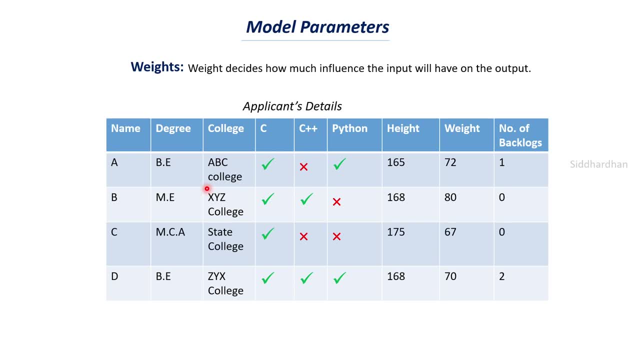 important, whereas some columns are not important. now let's try to understand which columns are, which features are important for making this prediction. so let's try to understand these columns individually. so first column is the name of the person. so now we can think logically. so the job offering that has been there is for the role. 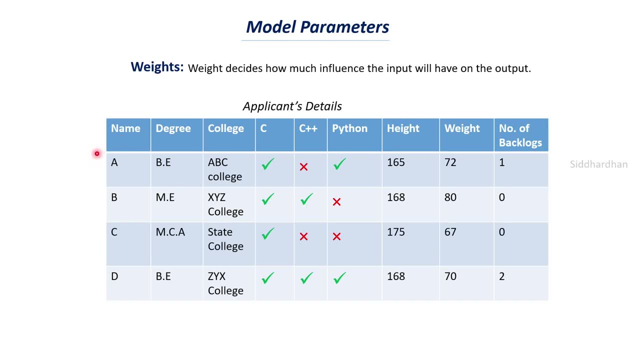 of software engineer. okay, and now let's try to see which columns are, uh, important for us. first column is the name of the person. so if we think the name of the person has nothing to do with whether they will get a job or not, right, so the person can have any name and their name does not. 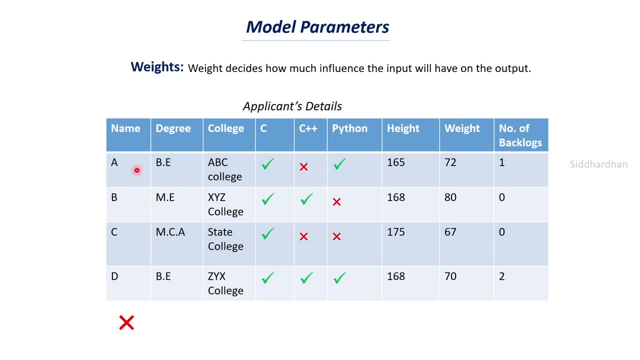 influence whether the person will get a job or not. so this particular column, this name column, won't be that much important for us, so, or in other words, it won't be important at all. and the second column is the degree of the person. so the first person, the person a, has 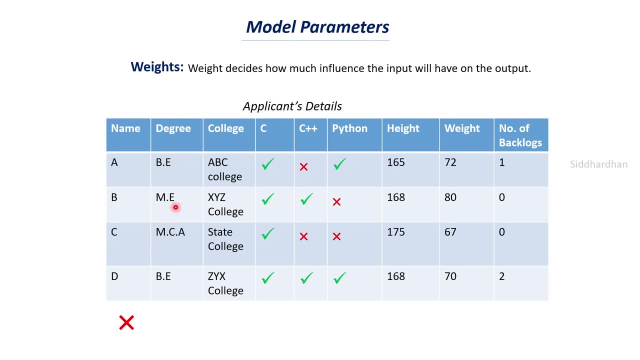 studied a bachelor of engineering, and the second person has studied- uh you know, master of engineering. maybe, uh, you know, in computer science or information technology. third person has studied mca and the fourth person has also studied b. now let's try to see whether the degree is important. 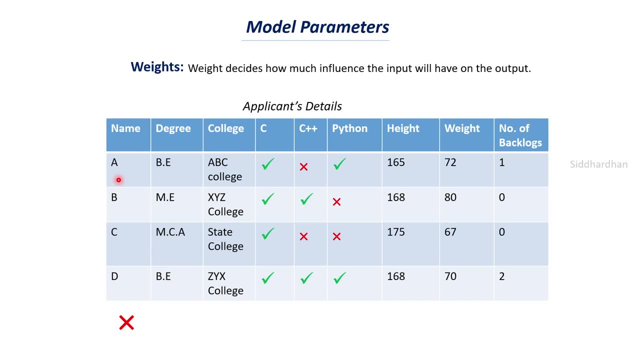 for that particular role. yes, we know that the degree or the educational qualification of a person to decide whether that person will get a job or not. so this second column will be very important for us. so this column is required for our prediction and the college they studied. 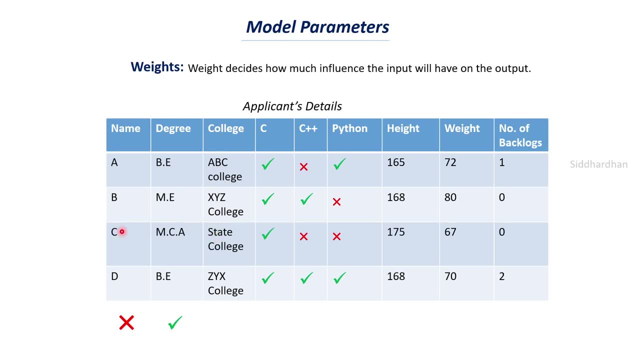 so, uh, you know, i've just uh named some colleges and we know that the college that they are studying will actually influence, uh you know, whether they would get a job or not. if the person is from a- you know, itr college, there is a high chance that that person will get a job, that particular job. 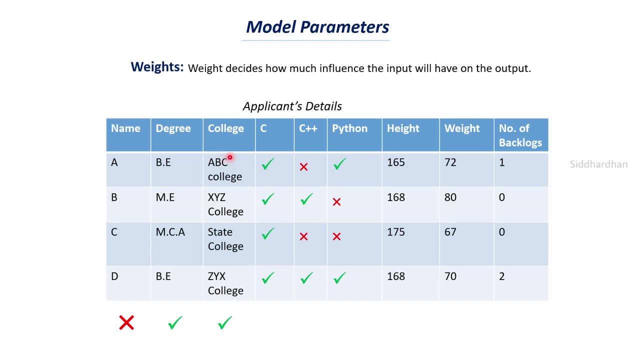 so it is obvious, right? so this particular column is also essential. and now we have the three programming languages, so for a software engineer, it's important for them to know programming languages, right? so these three columns will be will be important. so whether a person knows c, c, 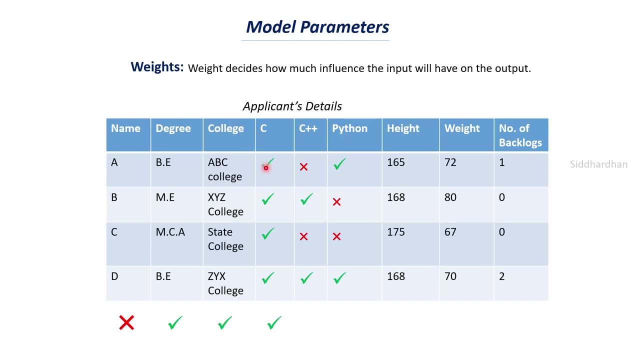 plus plus and python. so let's say that this tick green tick represents that the person knows c programming and x mark represents that that person does not know that particular programming. so in this case all the four people uh knows c programming and two people doesn't know c plus plus, and so on. 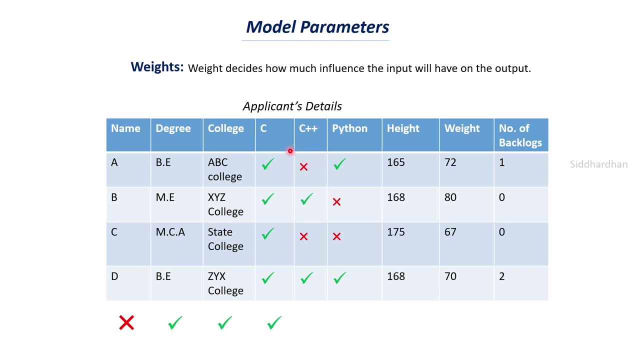 okay, so x represents the person who does not know that particular language. so these three columns for our prediction to determine whether the person will get a job or not. okay, so these three columns are important. now we have the height and weight column, so we can confidently say that the 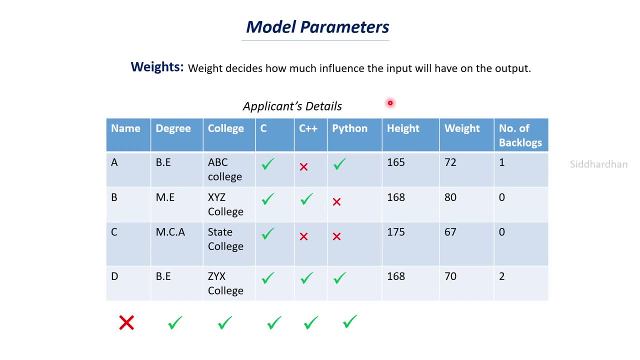 height and the weight of the person doesn't influence the that they are going to get the job right. so it is not relevant to that particular use case. so the height and weight of a person does not- uh, you know, influence whether a person will get a software engineering job or not. so these 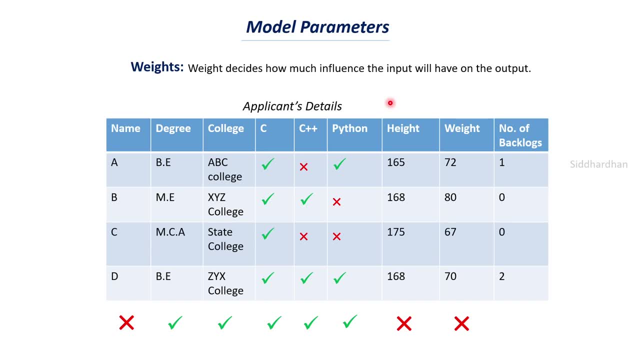 two uh columns are not required. and finally, the number of backlogs. so this is very important, right? more number of backlogs are. if a person has more number of areas, then, uh, it's most probably that he may not get a job, and if a person does not have any backlogs at all, then, uh, the chance or the 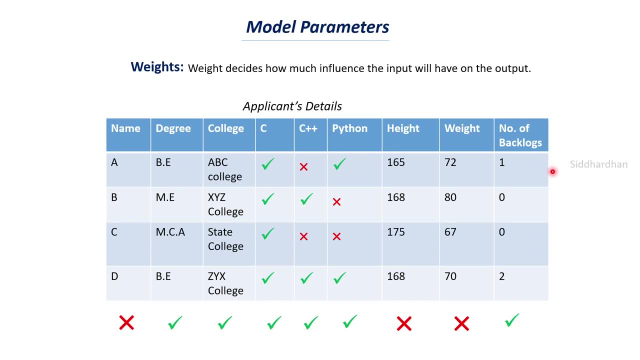 percentage that that person will get a job is really high, right? so this will be a very important uh feature for us. so out of these uh nine features, we have excluded the three features. one is the name name column, height column and weight column, and the remaining six features are important for 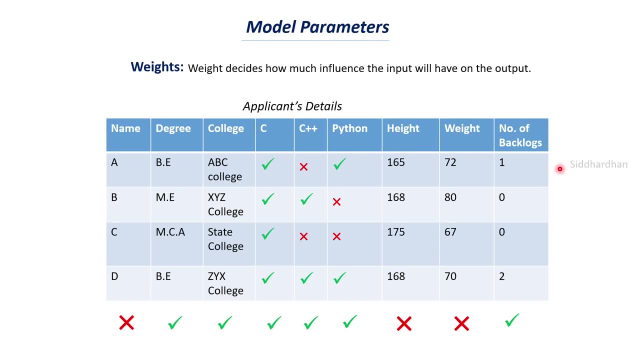 us to determine whether the person has- uh person can get a software engineering role or not. now we need to give a numerical value to emphasize the importance of these columns, and this is where weights will help us. okay, so we will assign some particular numerical value to this column. so, when it comes to name, height and weight, we know that. 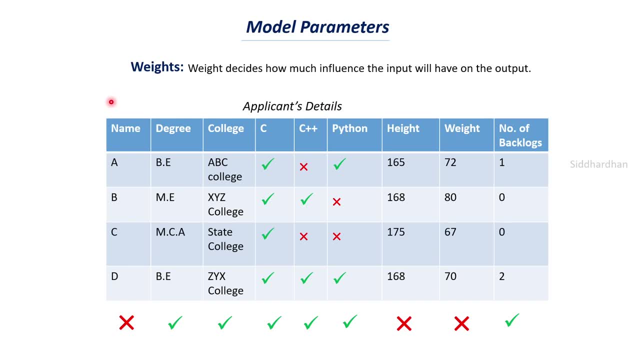 these columns are not important, right? so in this cases we can give the value of 0 to weight. okay, for name, height and weight we can give the weight value as 0 and different columns have different weight values. so each of these columns will have different weight values and it is not a common 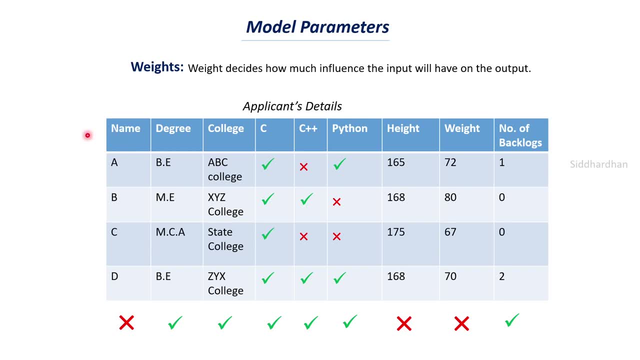 value. so if there are about nine features, you will have nine different weight values. and uh, and this weight value is not constant for different columns because we know that each column has separate uh, you know importance. so say, for example, the degree has a high weightage and the college also has some. 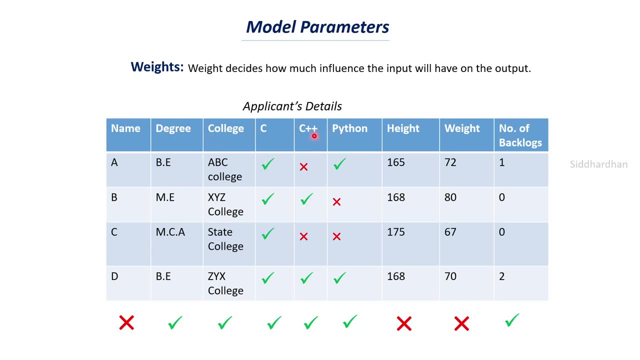 weightage and this programming. so these three columns as a high weightage, when it when we compare it to degree and college and so on, and number of backlogs. this number of backlogs has a negative impact on the job of the person. right, the person has certain backlogs, then, uh, we need to say that that person is not likely to get that. 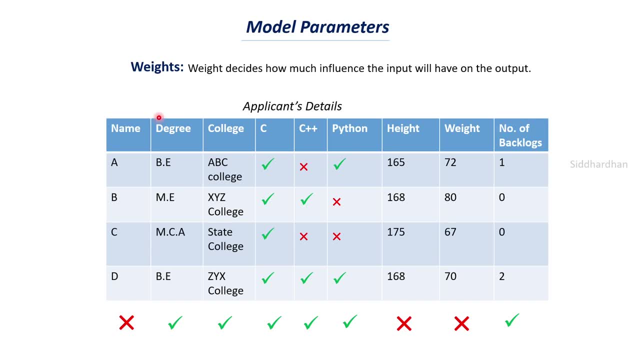 job. so in this case the weight will have a negative value. so the positive columns or the positive features will have uh positive weights. so the desirable or the favorable columns will have the positive weight values, the undesirable columns or uh. the undesirable column in the sense is the number of four years. so it will have a negative uh weight value. so that is one main. 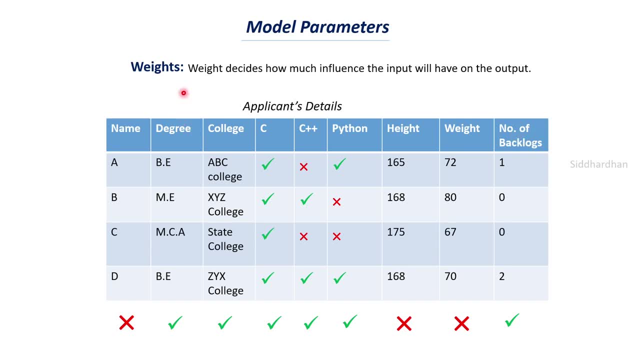 thing that you need to understand. so positive weights means that is a, you know, a positive result, and negative weight means there will be a negative result if we have the high number of values in that particular column. so that's one main important thing that you need to understand. so weight is: 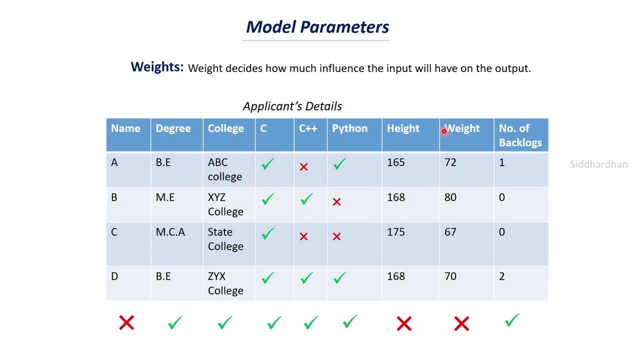 helpful for us to decide which column or which feature will influence the output. here. the output will be the- whether the person will get a job or not. okay, so this is the importance of the weight of a model. so this is nothing but the slope of the line that we are talking about. so here i have. 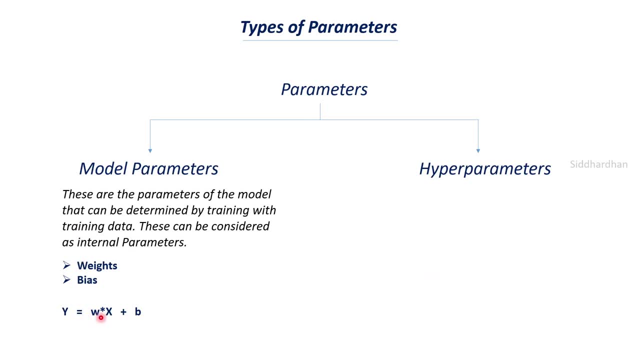 told you right, y is equal to w, x plus b, and this slope actually represents this uh, importance. okay, so in this case, the example i have taken is x represents the number of years of experience. right, so w will be the weight. so how much this particular column or feature will. 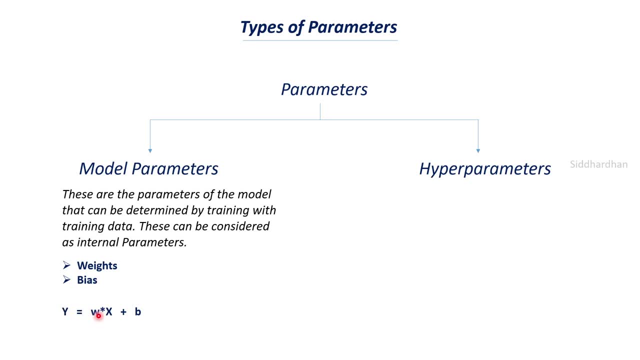 be helpful for us to predict the salary of the person. so that is meant by the weight of the model. okay, so i hope everyone is clear up to this particular mark. so, as i have told you, weight decides how much influence the input will have on the output. so the number of weights that we 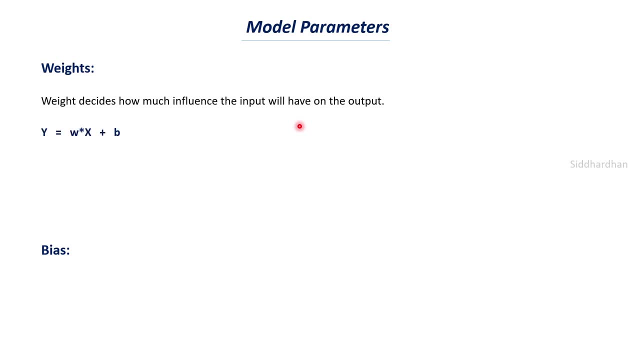 have is equal to the number of features that we have in a particular data set. so let's just say that y is equal to w, x plus b. so this is the equation of a simple line. okay, so in this case we have only one feature, which is x, and we have the output variable as y. so in this case, x represents 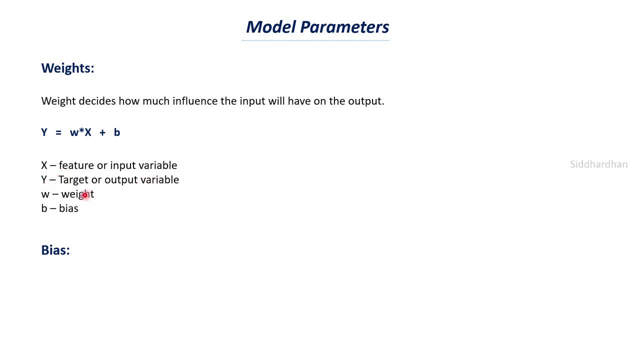 the feature or the input variable, and y can be the target or output variable and w can be the weight and b can be the bias. so you can also call this w as a slope and b as the intercept, when it is a linear model, when it is a simple line. okay, so in this case let's say that x represents the number. 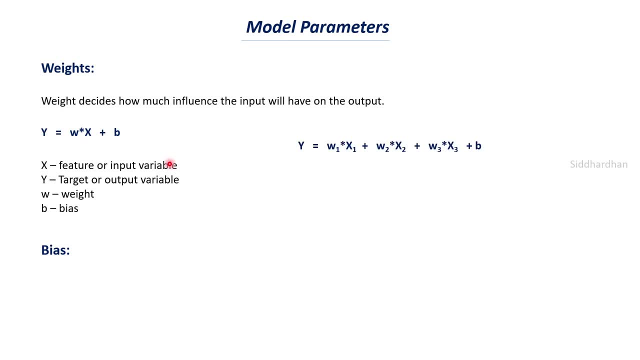 of features and y represents the salary of the person. now we may also have multiple features, as i have told you, right. so in the previous slide i have told you i have, you know, taken an example where we totally add about nine individual features, right? so similarly you can have. 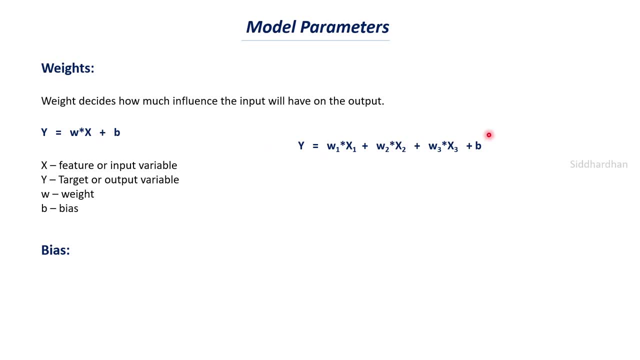 multiple features. so in this case we just add only one feature and in some cases we will have multiple features. so when you have multiple features, the equation of your model will look something like this: so y is equal to w1 into x1 plus w2, into x2 plus w3, into x3 plus b. okay, so 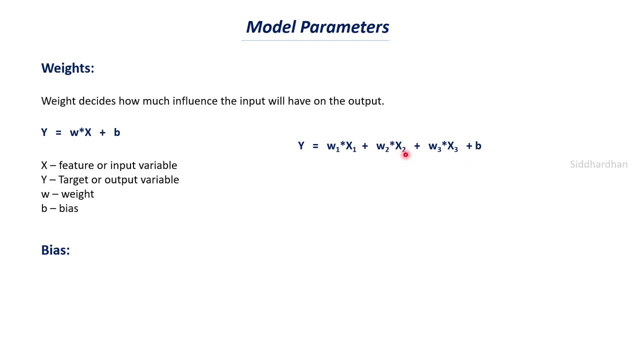 x1 represents it may represent the college from which they have studied, and x2 represents whether the person knows c programming or not. and x3 represents the backlog of a person. so this would be the equation when you have three different features, so the number of weights will be equal. 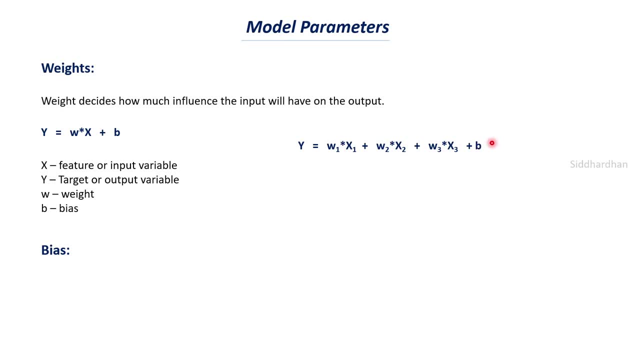 to the number of features that you have, and bias will be a- one single value. okay, so weight can be an array. so if you consider w1, w2, w3 and so on, all these weights can be considered as an array. okay, so, whereas b will be a single value, so you can. 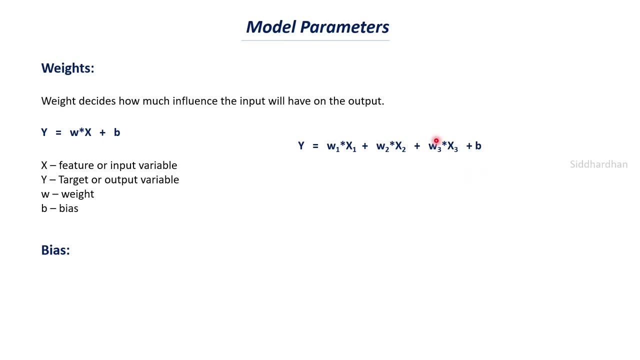 you know, include w1, w2, w3 together and you can call them as an array, but b will be a single value, bias will be a single value in this case. so the one main thing that you take to take a note of here is, in the case of a simple line, when you have a single feature, you will have only one. 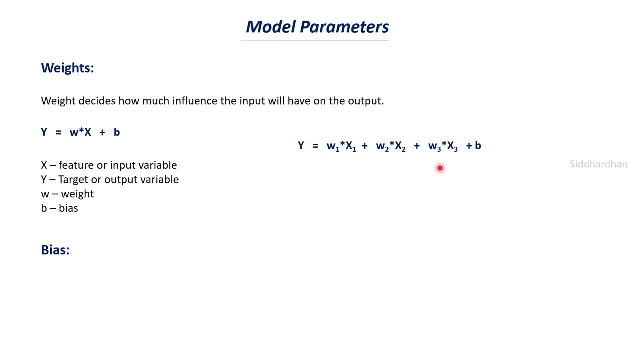 weight value or slope value, and when there are, you know, three different features, you will have three different. weight value: okay, and this weight value represents how much importance this x1 has on the target variable y. okay, and x2 and w2 represents the how much importance does x2 have on the target variable y? so if x1 represents, let's say that x1 is the 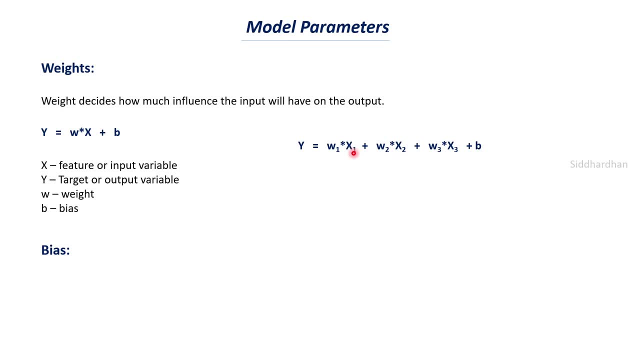 number of programming languages that a person know. let's say that a person knows four programming languages. so in that case, w1 would be a positive value because it is a desirable character, right? so the number of programming languages. and let's say that x3 represents the number of backlogs. 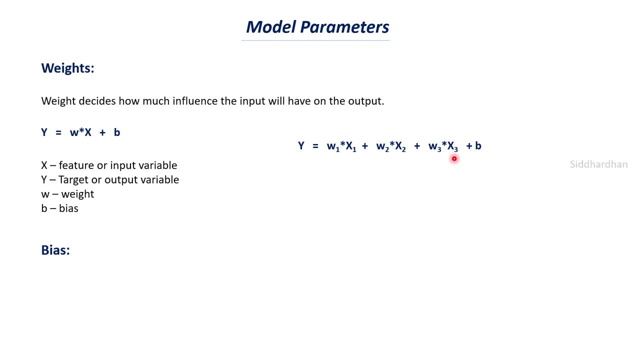 that a person have, so more the backlogs of a person, it is unlikely that is going to get a job and hence we can say that w3 will be having a negative value. so we can have both positive values and negative values for the weight of the model. so that's another main. 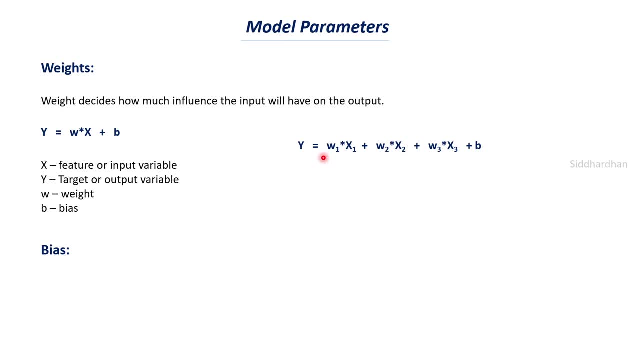 thing which you need to take note of. so that's it about weights of the model. now let's try to understand about the bias of the model. so you can call this bias as the offset value. okay, so the other name for bias is offset and bias is the offset value given to the model bias is used to. 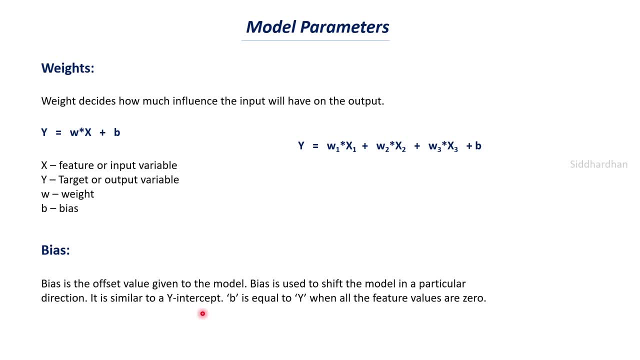 shift the model in a particular direction and it is similar to a y intercept in a simple linear regression model, and b is equal to y when all the feature values are zero. okay, so this is, uh, you know, a definition and a detailed description of bias, and let's try. 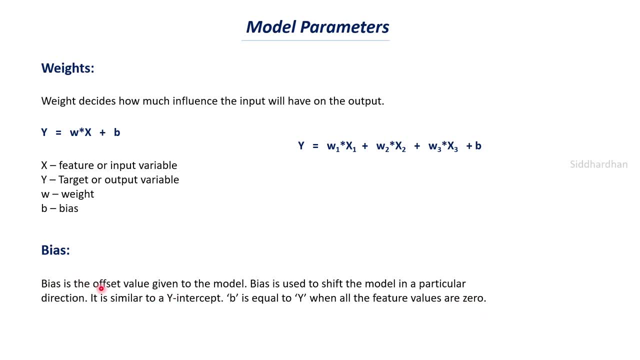 to understand about what is meant by this bias. so, as i have told you, it is an offset value of the model. so, as you can see here, both of these models have some bias value, which is b right, and it is used to shift the model in some particular direction. so i'll explain you what. 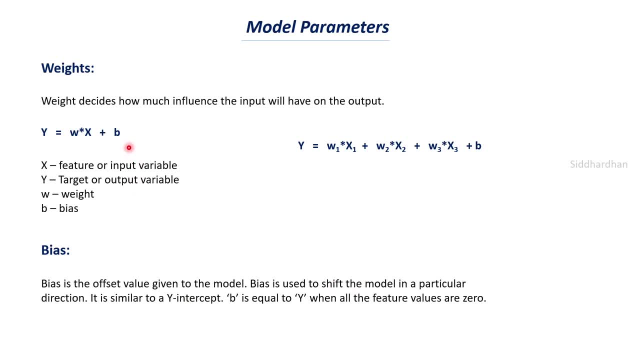 this exactly means- and we can call this as y intercept. so in my previous videos of linear regression i have explained you what is meant by this y intercept. i'll also give the you know link in the description where i have explained you about linear regression. so if you have some, 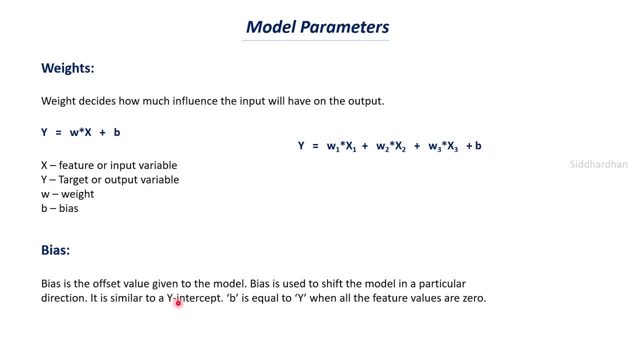 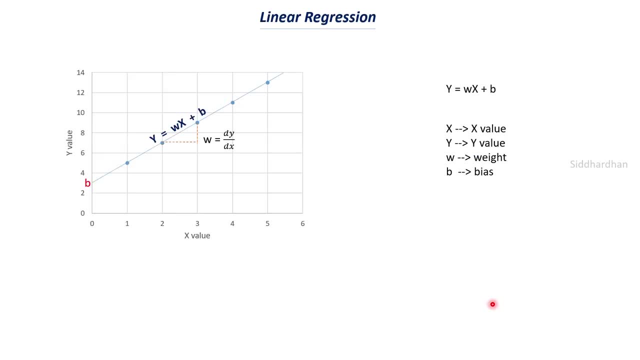 doubts, you can check that as well. so this bias is similar to the y intercept that we have, and b value will be equal to y when all the feature values are zero. now let's try to understand this with an example. so we know that the equation of line is: y is equal to mx plus c, and, as you, as you, 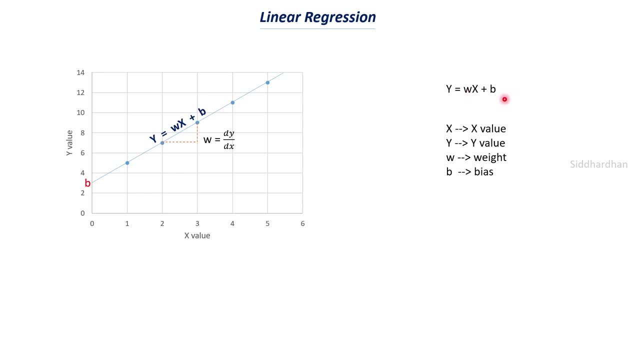 know i have replaced the slope value, the m value, with w and intercept value with bias b, right. so x represents x value, y represents y value, w represents weight and b represents a bias. so this will be a particular line. for this particular line you will have a particular 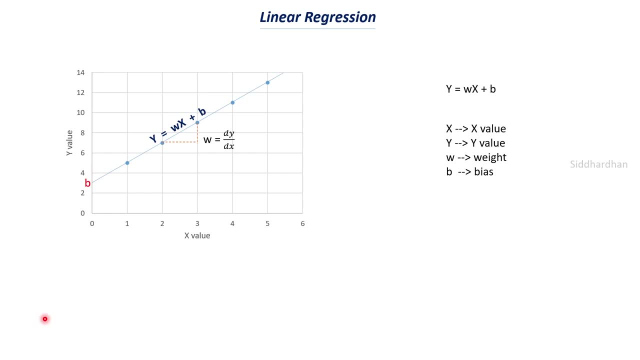 value for w and b. if you take a different line, so i'll just, you know, draw a different line here. so if you have a line like this, this line, so let's, let's say that this is a straight line. so this line will have a different slope value, different w value and different intercept value. and let's 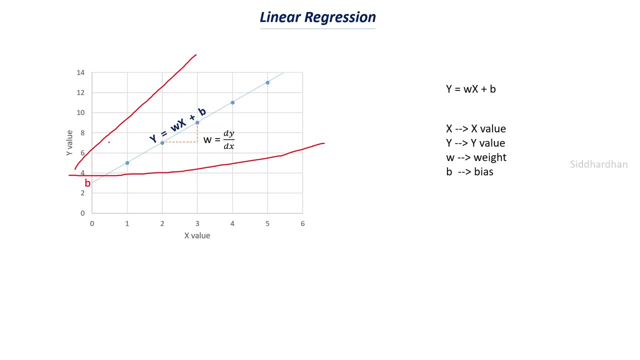 say that we have a line like this, so this particular line will have a different slope value again, a different weight value. okay, so now what happens is so sometimes, if you change the slope, the orientation of the line will change. okay, so slope is nothing but dy by dx, dy by dx. in the same sense, when the x value changes by a particular unit, what will be? 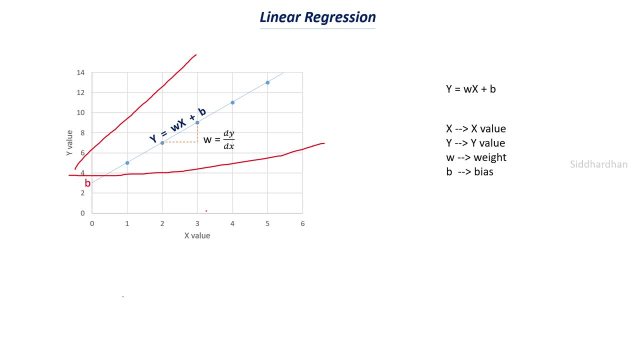 the change in the y value. let's say that, uh, here the x-axis value is 2 and the x-axis value, the second x-axis value, is 3, and if the x-axis value changes from 2 to 3, what will be the change in the? 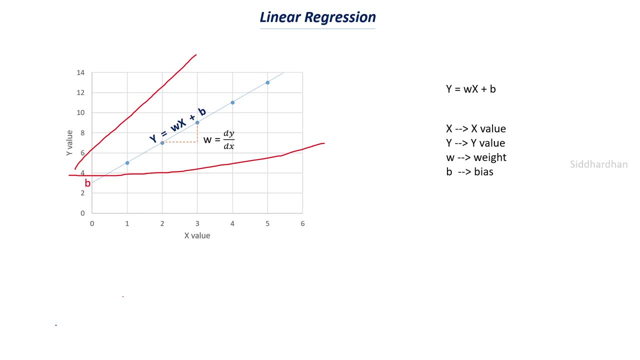 value of y, so that is called as the slope of the line. so we, everyone of us of us, knows this right. so if you are not clear about this, watch, kindly watch- my linear regression video. so it will, it would make a clear sense to you. so, as i have told you, so slope is nothing but the change of value in. 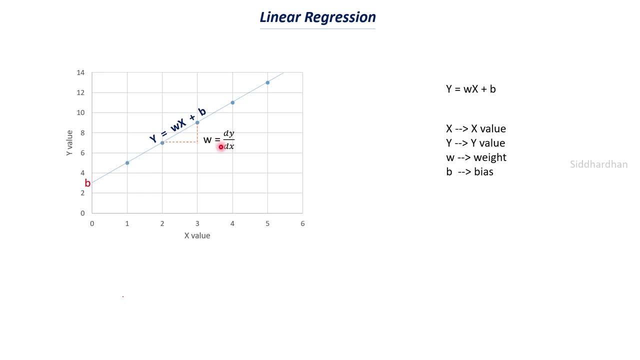 y when x changes. so if you change the slope of the line, if you change the slope of the line, your orientation of the line will change, okay, so if you change the slope value, you will get a line like this. so let's say that we get a line like this, so this line will have a different slope and this: 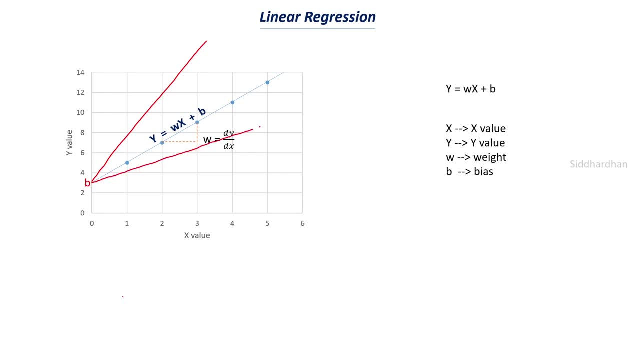 particular line will have a different slope, and if you have a line like this, this will have a different slope. so changing the slope of the line or changing the weight of the line will change its orientation. so that is called as the weight of the line, and then we have the bias. 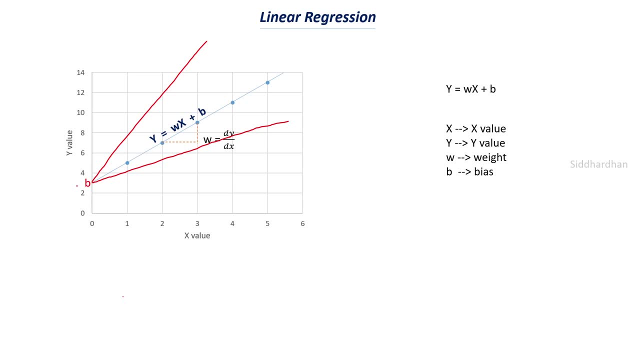 so bias is this particular region. so what is the distance between this particular point from origin? okay, so in this case, you can say that this particular value is three. right, so we have two, one, four as coordinates and, uh, this particular line starts from this point and this represents 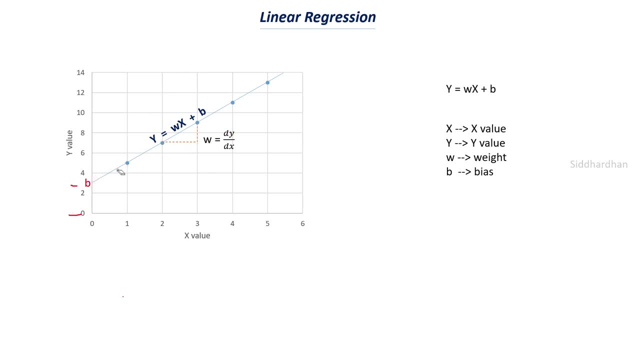 the bias of the line, so this is also called as the y intercept. okay, so whenever you change the slope of the line, your orientation changes, but you cannot change this particular position of the line. here the line starts from three and no matter how you change your slope, your uh position of this particular line won't change. so it will start from this point. 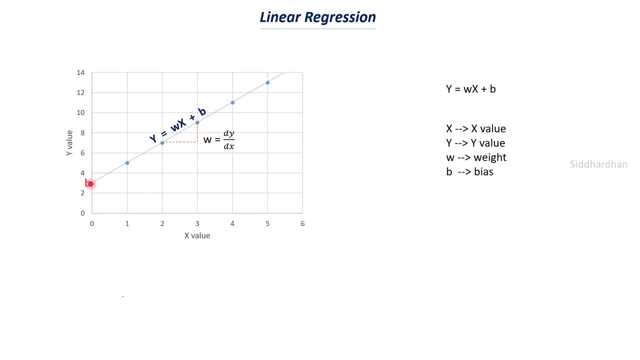 exactly three. and if you want to change this particular uh intercept value, you need to change the value of c, right? so that is why we have this bias. so if you change the bias value, let's say that, uh, we have a bias value as a six. so in that case what will happen is that if you change the 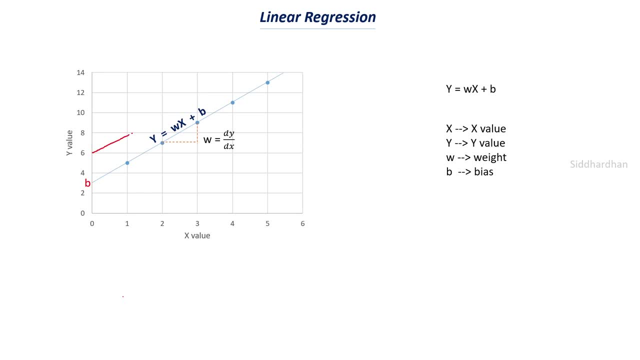 slope. your line will start from this particular point and it will be looking something like this: okay, and the slope will be the same in both the cases. if you have the same value for w and if you have, uh, the intercept value or the bias values as four, your line will changes. sorry, 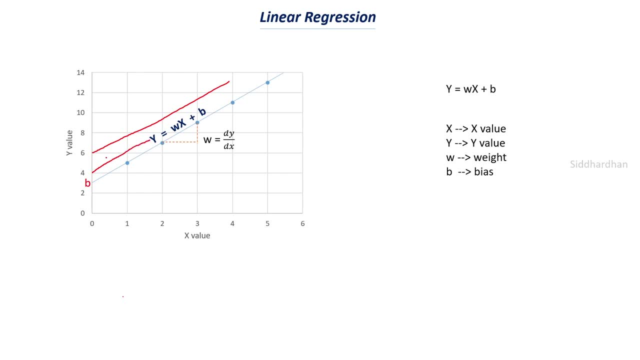 your line will start from this particular point. so this is the importance of bias value. so sometimes we need to uh shift this particular line in the upward direction or lower direction. so in case you have a intercept value as two, your line will start from here, right? so, no matter what, uh, you know. 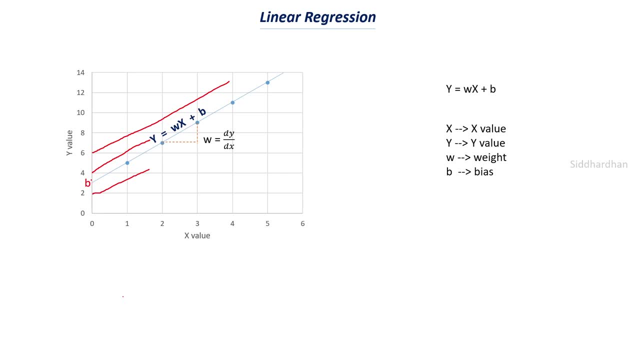 much you change your slope, your this particular point won't change. so if you want to change this particular point from where your line starts, so in that case you need to change the bias value or intercept value. so that is the importance of this bias. okay, so changing the values is really. 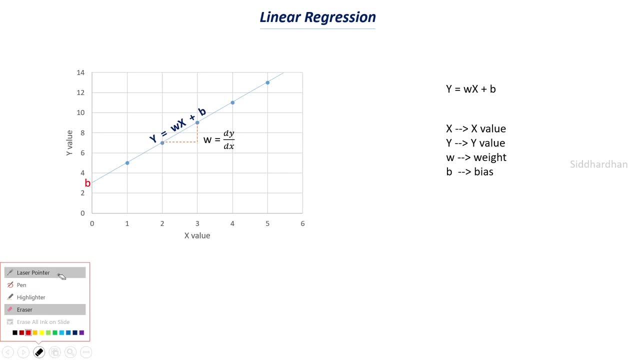 important for us when it comes to machine learning, as it is nothing but the optimization techniques to find the better values. so this is the importance of bias value. so you can also, you know, easily find this intercept value. so intercept value is nothing, but, uh, let's try to. 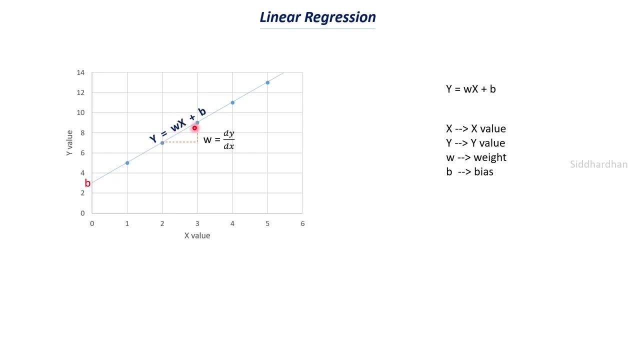 put the value as a 0 for x. okay, so let's try to take this equation and let's put x value as 0. so what will be the this equation when x is 0? so w into x, which is w into 0, will be 0 and y will be. 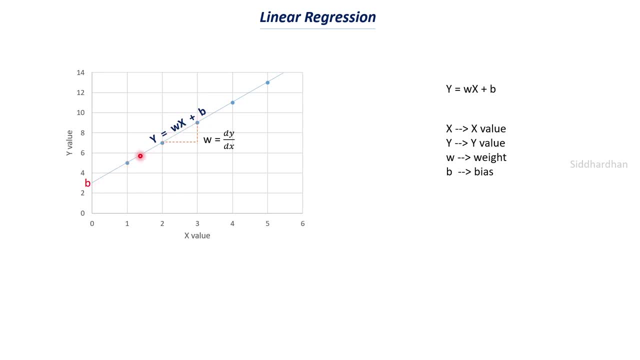 equal to b right. so b is nothing but the value of y when x axis value is 0. so now you can see this equation. so let's try to take this particular point, so let's try to find what is the coordinate of this point. so this coordinate of this point is nothing but b, 0 comma, b right, where 0 represents. 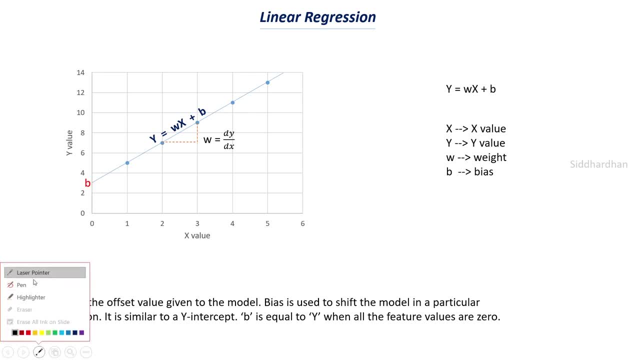 the x-axis value and b represents a y-axis value. i'll just write it here. so this particular point: b represents 0 comma, so 0 comma b, or it's 0 comma 3 to be exact. okay, so i'm not good at writing. so. 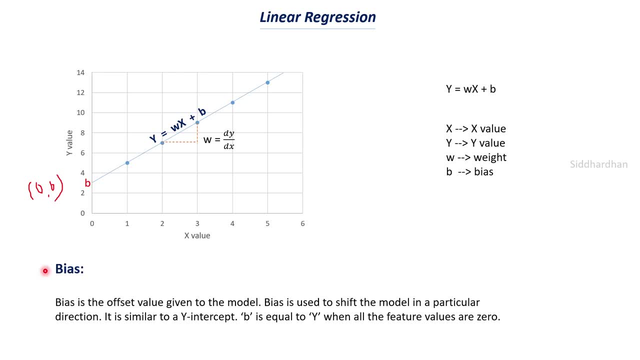 just, uh, tolerate this. so it's 0 comma b. so this 0 comma b represents this slope of the range. so you can also say in different words that bias is equal to y when x is equal to 0. okay, so that's what i am. 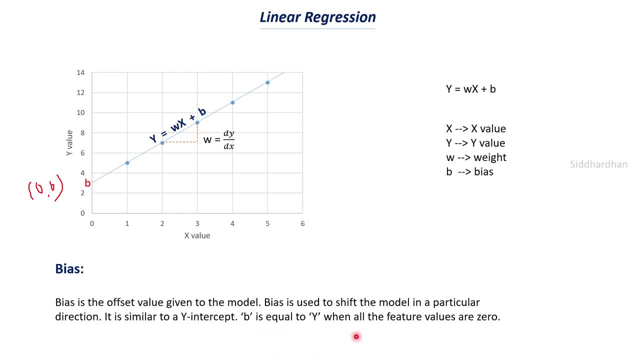 given. in this particular equation, as you can see here, b is equal to y when all the feature values are 0. here feature value is nothing but x, right? so that is all about weight and bias. so bias is the offset value that we give to our model. so this: 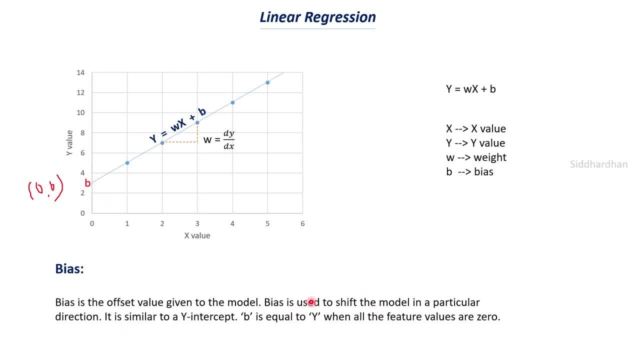 is that particular offset value and this bias value is used, used to shift the model in a particular direction. so in this case, when it comes to a linear regression, it is simple for us to shift the model in the upward direction or the downward direction. so we want our 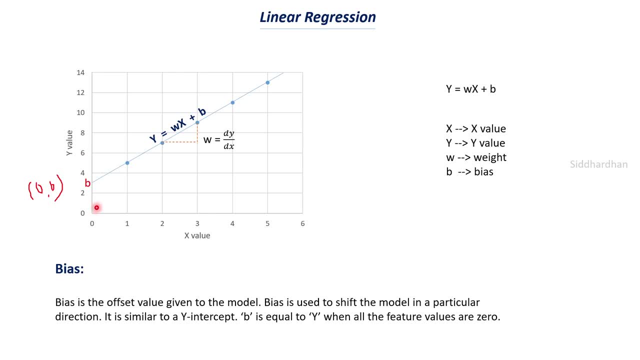 line above this point or below this point and so on. and there are models like sigmoid curve. so in in the, in that case the sigmoid curve will be shifted in the left direction or the right direction if we change the bias value. so for a line when we change the bias. 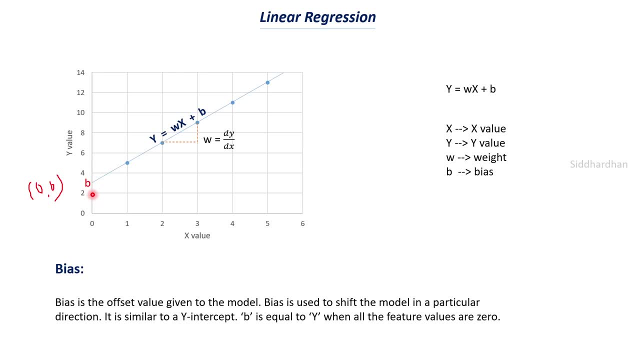 value, your line will move in the upper direction or lower direction. okay, so the line will shift in the upper direction or lower direction. but when it comes to a sigmoid curve, your curve will shift in the left direction or right direction when you change the bias value. so that's a topic for 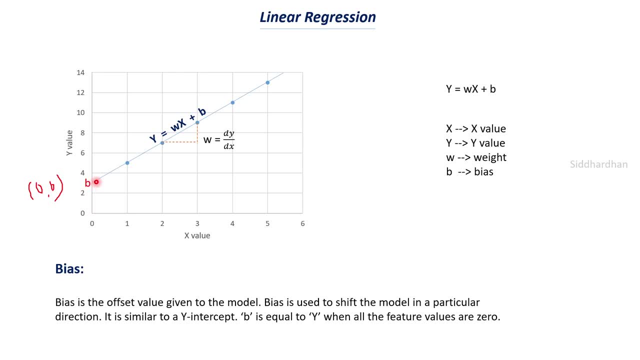 discussion in some other video. but just try to understand this: when it comes to linear regression, change the direction of the line- sorry, the this particular point in the upward direction or lower direction. okay, so that is all about bias. so bias is the offset value and it is used to shift the. 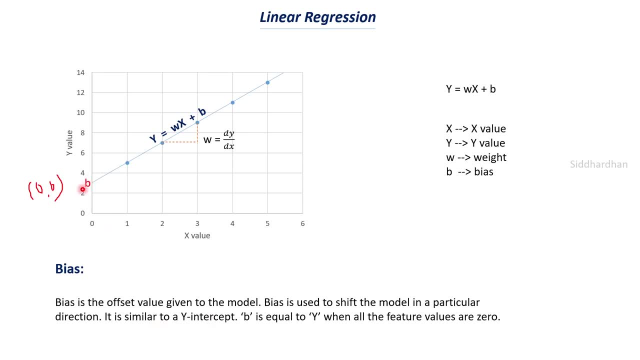 direction of the model. okay, and it is similar to the y intercept. so this is nothing but the y intercept. y intercept in the sense, what is the value of y when the value of x is zero? so that's what i have given here. so this is all about, uh, the slope and intercept of the model, or the weight, or 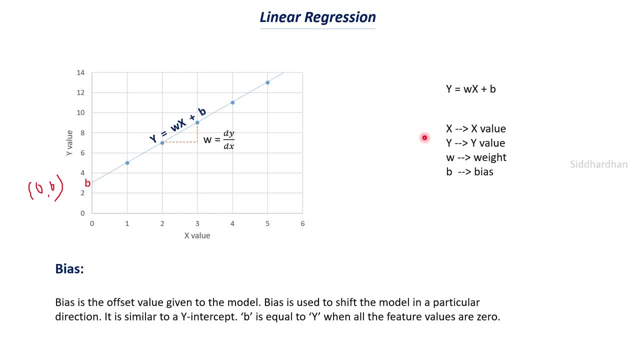 the bias of the model. okay, so these two parameters are else called as the model parameters, and this model parameters differs based on the data that we have. if we use different uh data, then we will get different values for weights and biases. okay, so this is all about uh model parameters. 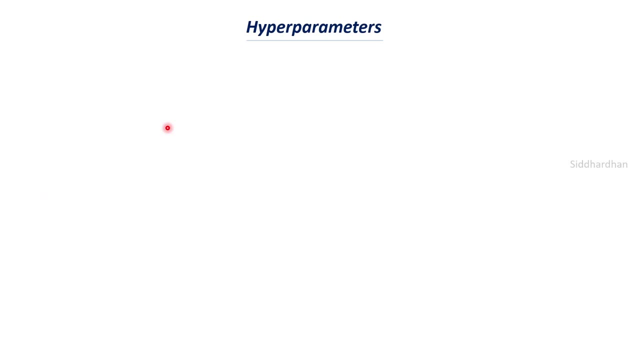 and the next parameters that we have is hyper parameters. as i have told you, uh, the two hyper parameters that we have are learning rate and number of epochs and, as i have mentioned earlier, we will try to uh reiterate the model with the data. so we will. 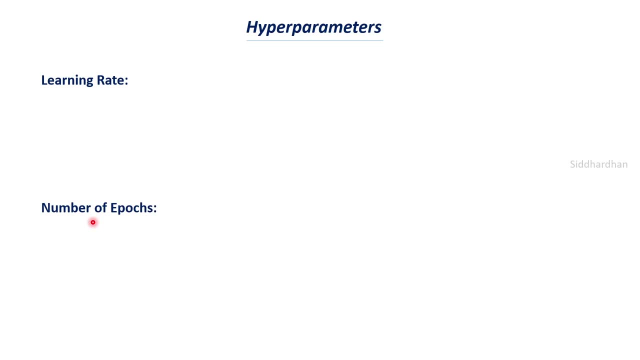 try to fit the model again and again with the data. let's say that we have uh under deterioration, so under iterations, in the sense we want our model to go through the data under different time in order to find the best weight value and the best bias value, so that our model can make better. 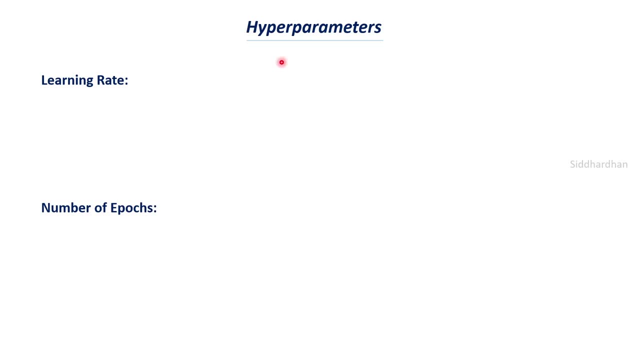 predictions okay, and hyper parameters are helpful for optimizing the model. optimization is nothing but a technique which is used to make better model parameters so that we can make better prediction. so now let's try to understand about the learning rate and the number of epochs. so the learning rate. 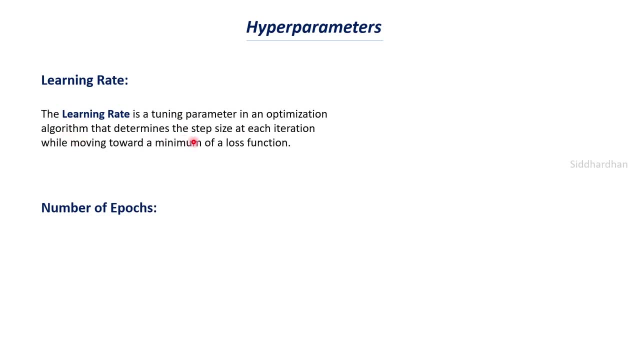 is a tuning parameter in an optimization algorithm that determines the step size at each iteration while moving towards a minimum of a loss function. so this is the definition of learning rate. so just look at the word tuning parameter and optimization algorithm. so what happens is we need to change the values of weights and bias. 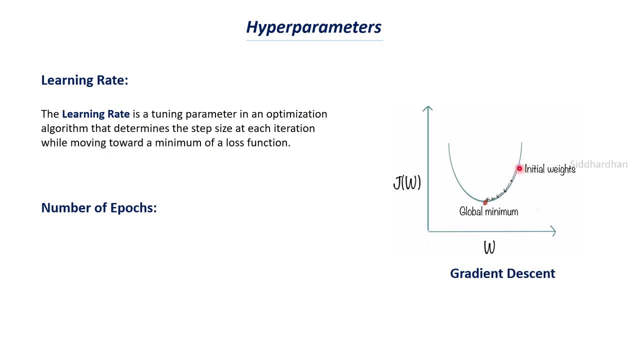 right in order to get a better value. let's say that this particular point represents the initial weight. so we are starting from this initial weight and let's say that this initial weight w is not a good parameter, so that that particular weight value is not giving us good, good prediction. so 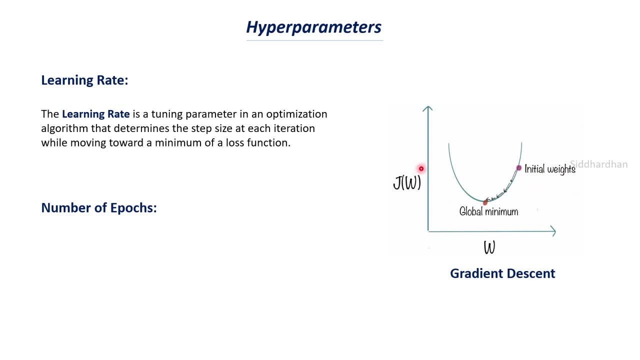 that particular weight will have i loss function. so if you don't know what is meant by a loss function- and i have already made a video on loss function- i'll also give that particular video link in the description. so do check that out as well. so if a model is not performing well, then 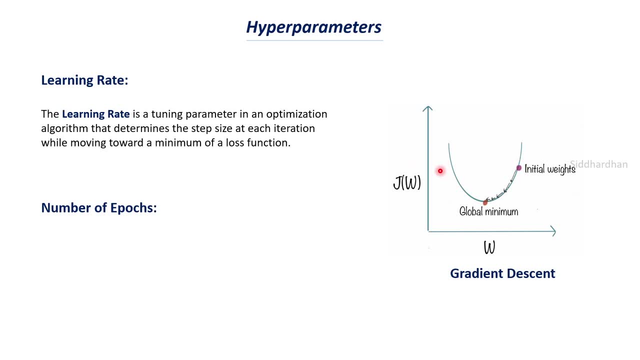 it will have a very high loss function. if a model is performing well, if it is making accurate prediction, in that case the loss function value will be very- you know, very- low. it will be zero and so on. okay, so i loss function value means, uh, the model is uh not working properly and low loss. 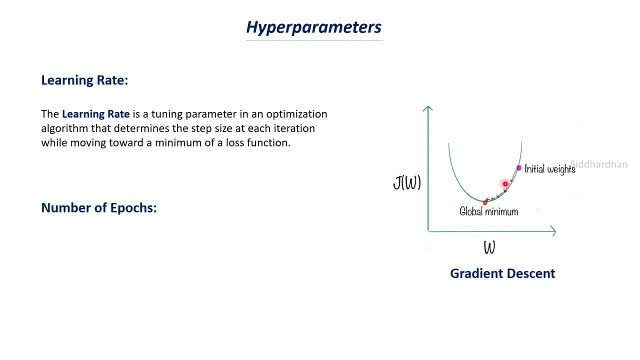 function value means the model is working properly. so from this point we need to reach to this particular point where the loss function value is minimum. okay, so what we will do is we will repeatedly change the weight value to see what will be the optimum parameters, or optimum parameter value or the weight value, so that we 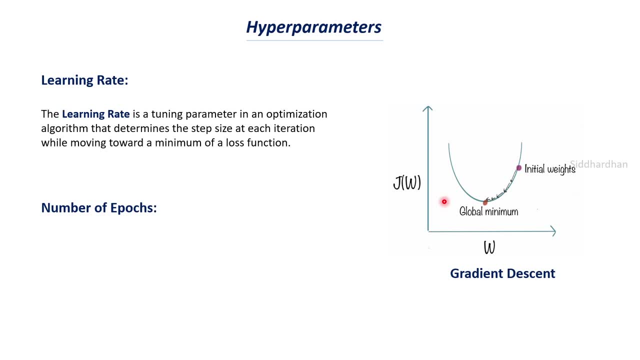 can get a minimum loss function okay. so the idea here is to minimize the loss function. so j of w represents the loss function, w represents the weight of the model. so we need to change the weight of the model so that we get a minimum loss function. so minimum loss function means accurate. 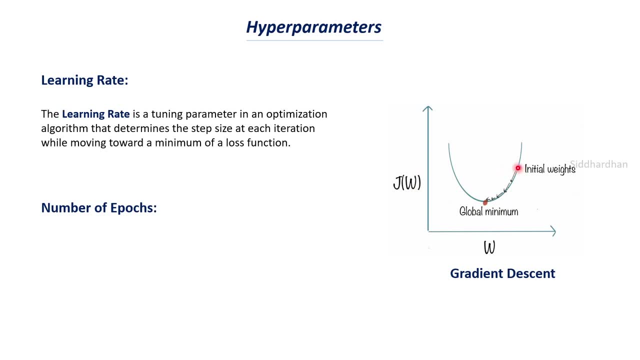 model. right, So we start from this particular point, a particular initial value, and we will try to change this value and so on, so that we can reach this global minimum. okay, so global minimum is the point where the loss function value is minimum and there is a change in the weight value. right, so this change in the weight value can be, let us say that the weight value is 10. okay, so let us say that we have a linear regression model and this equation of this linear regression model is: y is equal to 10x plus 3. 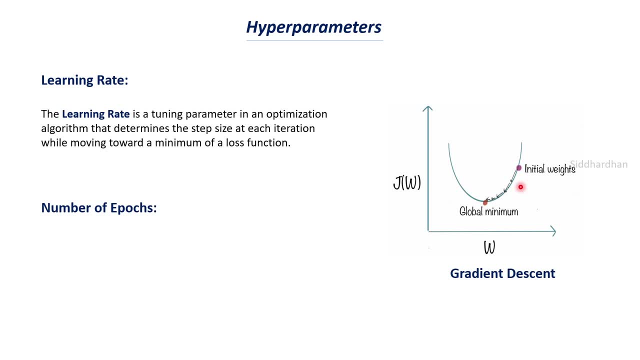 where 10 represents the weight and the 3 represents the bias value. now we need to repeatedly change this weight value. let us say that we change the weight value by 1 in each step. so this represents this: one direction represents one step, the next direction symbol represents another step, and so on. so we need to come in this direction right. so each step will reduce your value or it will reduce the value of our weight by 1 unit. so if you start from 10 unit, so each step you will take will reduce your value by 1 unit. 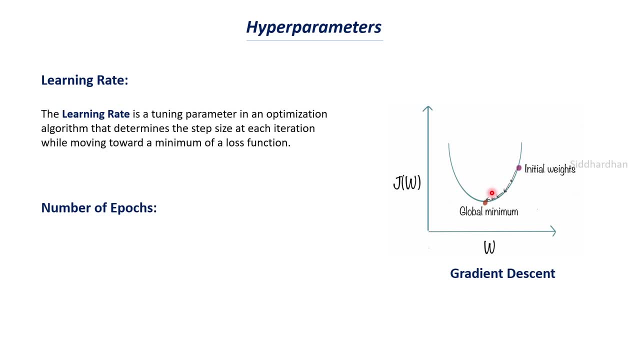 So the second iteration when you do, your weight value will be 9, so that represents your linear equation will be: y is equal to 9x plus 3. and the next iteration, again, your weight value will be reduced by 1 unit. so in this case your linear regression equation will be: y is equal to 8x plus 3, and so on. so in this case the change that you are giving your to your model is 1 unit right, and this amount of change that you are giving is called as the learning rate. so often we want to give that much learning rate. so the learning rate that we will give will be in the range of 0.01.. 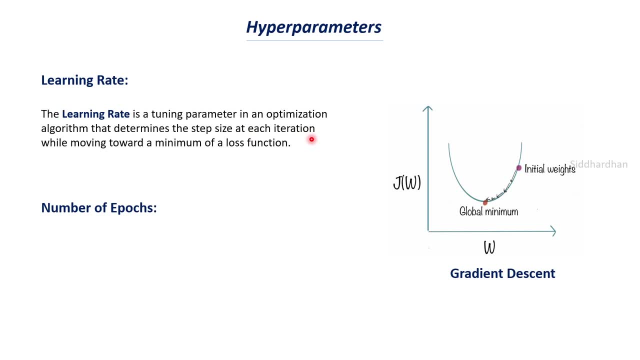 Or 0.001 and so on, and it completely depends on the data set that we have and it depends on the magnitude of the weight that we have. so if you have a weight value around 1000, in that case you cannot use a learning rate as 0.01, right? so it would be very tedious in that case. so it depends on the magnitude of the weight that you have and it depends on the data that you have. so this is called as the learning rate. so in each iteration we will try to change the weight value and we will try to see whether the loss function is reduced or not. so the change that we are imparting to the weights is called as the learning rate. 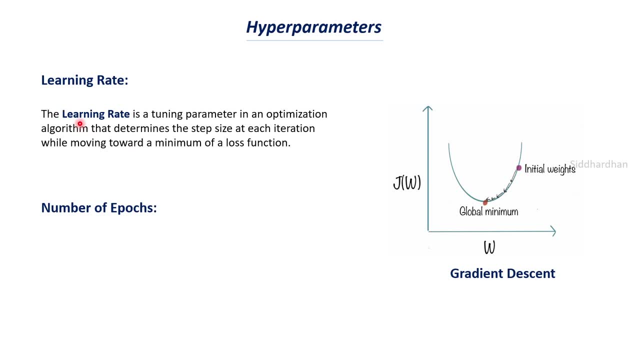 So how much value, or how much change in the value that we are giving to our parameters. so now read this definition again. so the learning rate is the tuning parameter in an optimization algorithm. so that determines the step size. so step size is nothing but the change that we are imparting at each iteration while moving towards a minimum of a loss function. so the minimum of a loss function represents the global minimum where the loss function is minimum. so whenever the loss function is minimum, that means the model is making accurate prediction. okay, so this is an example of a gradient descent. so this represents a gradient descent. 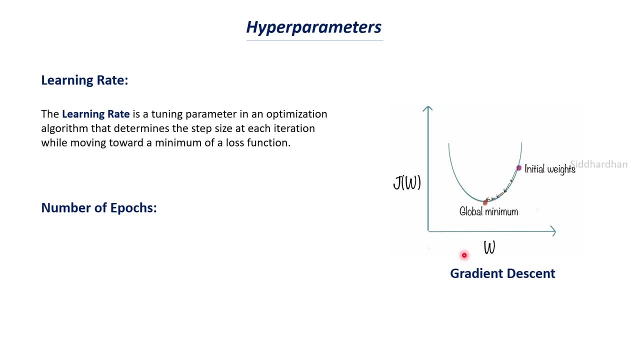 algorithm and the gradient descent is an example of a optimization algorithm. so in the upcoming videos we will discuss in detail about gradient descent. and if you don't understand about gradient descent is completely fine, i'll make a separate video on this gradient descent- and it is a very important concept in machine learning. so in several models we use gradient descent as our optimization model. so it is very important for us and i'll explain you clearly what is meant by this gradient descent. for now, try to understand that learning rate is the amount of the change that we are imparting to the model in each step of the model. 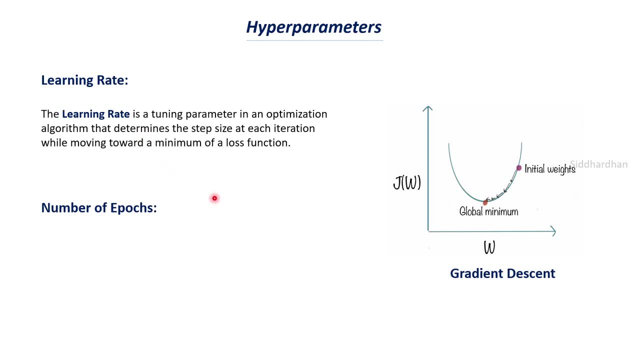 the training process. okay, so this represents the learning rate. and now we have the number of epochs. so number of epochs represents the number of times the model iterates over the entire data set. okay, so let's say that we have 100 iterations. so in that case what we will do is, in each 100 steps, we will try to change, we will try to change the parameter value by some certain amount. so in that case we will give some particular learning rate value. and number of epochs is like the number of iterations. so it is very simple: the number of times you want your model to go through the data set. 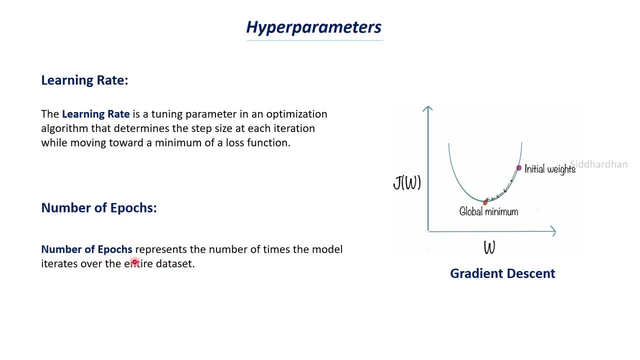 so this represents the number of epochs and you can give any values for your epochs, so you can give 100 iterations or you can give 1000 iterations and so on, and it also depends on the data that we have and the model that we are choosing and so on. okay, so if you give a very high number of epochs, there is high chance that your model will overfit, and if you have a very low number of epochs, then there is a chance of underfitting. so we need to find the optimum value of this number of epochs and learning rate, and not having a proper learning rate or the number of epochs will result in 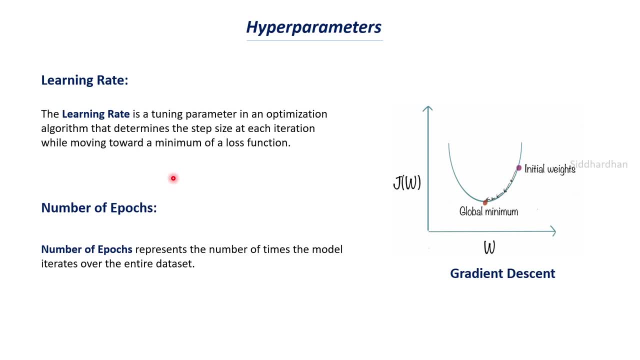 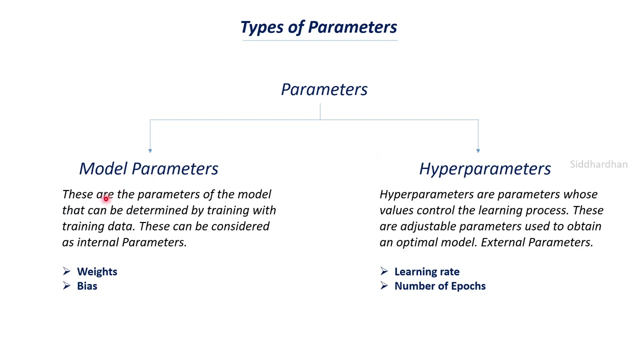 either underfitting or overfitting. so we need to find a proper optimized value for learning rate and number of epochs, and for this we use some techniques called as gradient descent and so on. okay, so these two are called as the hyper parameters: the learning rate and number of epochs. so that is for this particular video. so i hope you have understood about the model parameters and hyper parameters. so it is the same slide that we had before. so now you can see this, or you can read this definition again, and you will, you would have gotten a better understanding. so model parameters are: 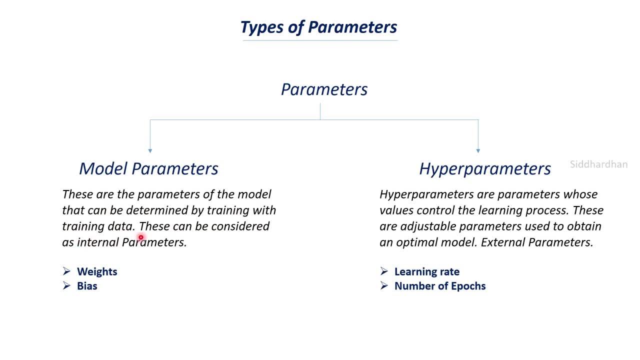 the parameters of the model that can be determined by training, with training data, and these can be considered as internal parameters, such as weights and bias. okay, so we know that once we train uh the model with the data, we will get this particular parameters and hyper parameter is outside the 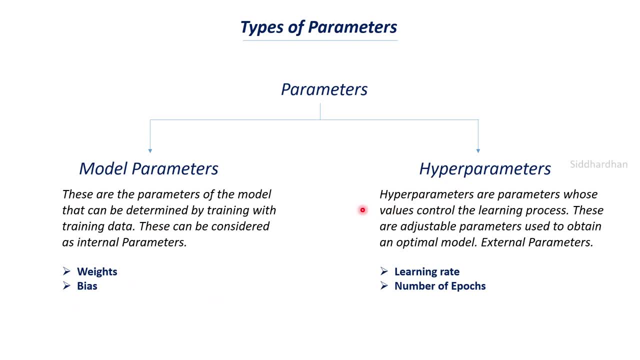 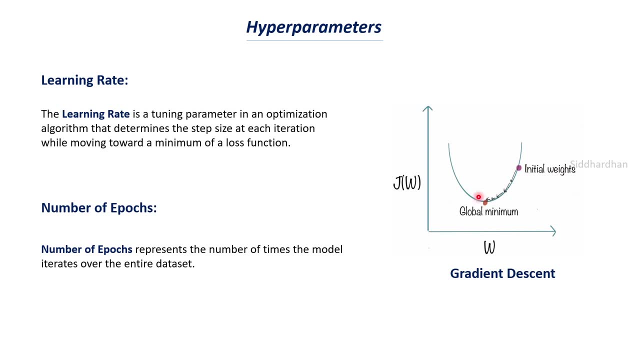 outside the model. so this hyper parameters are all about controlling the learning process, right? so we have a learning process where we will try to optimize the values of weights and bias. so this learning process is controlled by the hyper parameters, values such as learning rate and number of epochs.